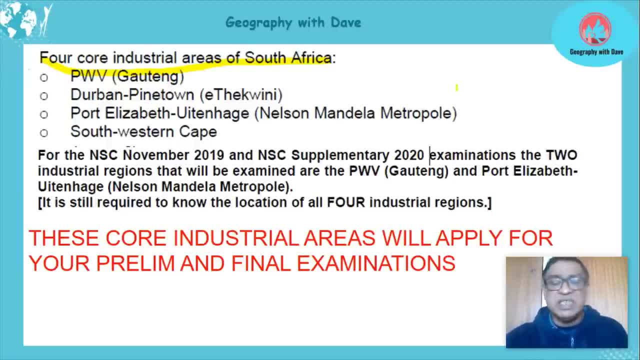 the majority by far economic activities. These are compared to other areas in South Africa. These are highly developed industrial regions with strong economic output, etc. okay and uh, we're looking at them. they're four regions: the pwv, all right, that's here. we're durban pine town, as people also say, itekwini port, elizabeth, euton egg- that's also. 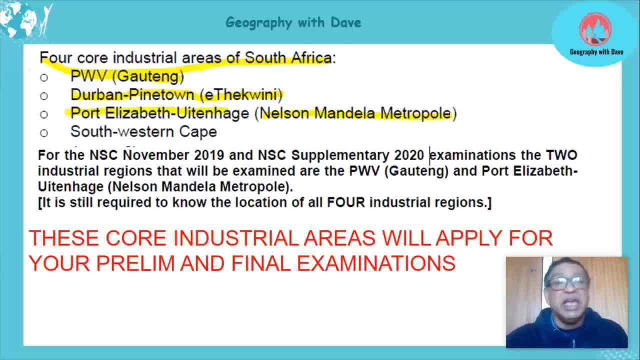 known as your nelson mandela metropole area- all right, and the southwestern cape. these four are huge. okay, now learners. there seem to be some confusion, of course, exam guidelines and your teachers would have explained this to you, but some of you are still. of course, it's important to have 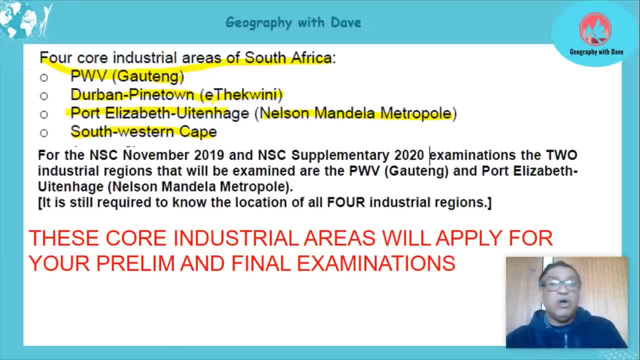 the exam guideline, which was from 2017. okay, and in the guideline it says: for nsc 2019 and supplementary 2020, the two industrial regions that will be examined are the pwv and the port elizabeth euton hague area. all right, it says that 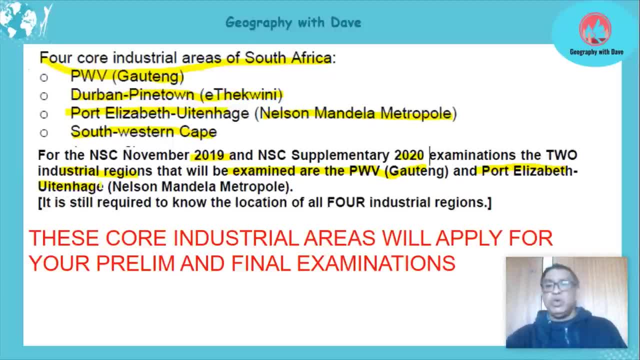 there now, just to let you know. i'm sure you will know, uh, this already, because you've got excellent educators and you are excellent yourself. okay, these core industrial areas will apply for your final exams. okay, so it's the same. so maybe the 2020 exam or the 2017 exam guideline. 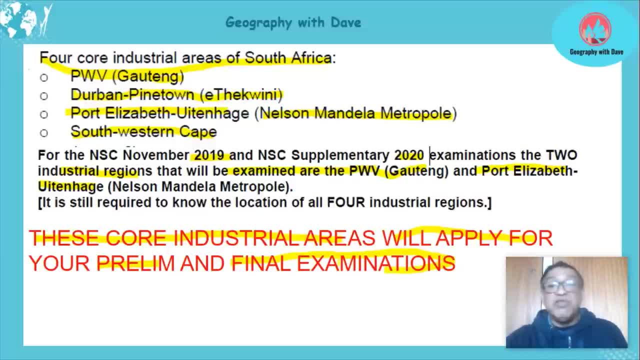 did not mention this. it will apply for end of the year, okay, and it says: although we're focusing on this, you still need to know the location of all four industrial regions. okay, where are they located? all right, so that's important, but your main focus is on the pwv. 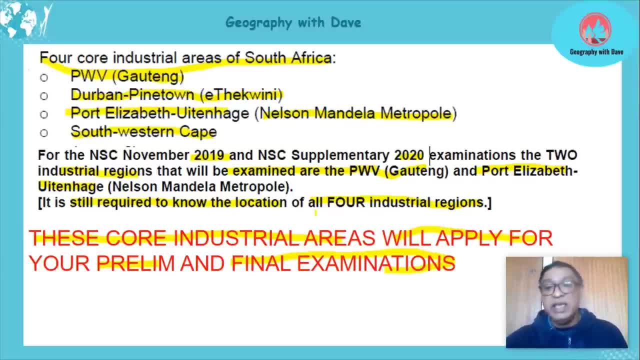 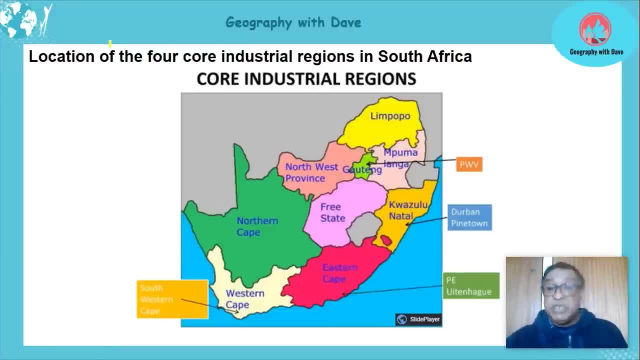 and the port elizabeth euton hague area. okay, let's go on now. we said we need to know the location of the four core industrial regions in south africa. now we have one which covers gauteng down here. that's your one core industrial area that we are going to deal with in more detail. 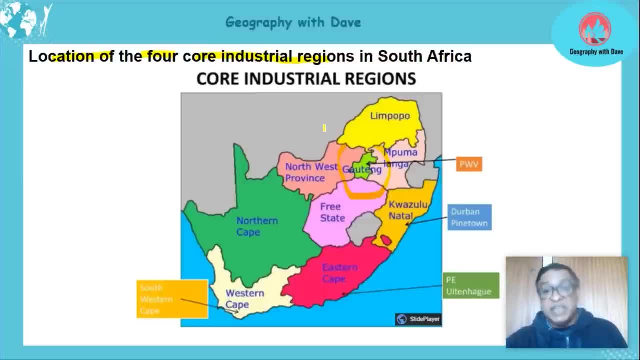 all right, it's known as a pretoria, also known as gauteng, and in short, it's the pwv. then in kwazulu natal, around the region here, we have the durban pine town core industrial region. okay, and then, of course, that's the second. 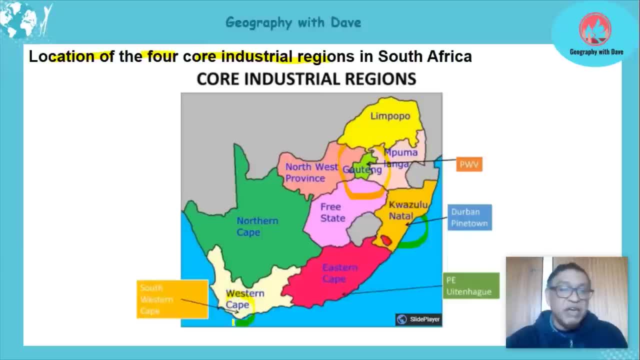 largest and the third. one third largest is we have in the western cape and the southwestern cape core industrial region that's found in the western cape, and then the last one of the four we have is the port elizabeth euthan egg area or in core industrial area that's found in the eastern cape. 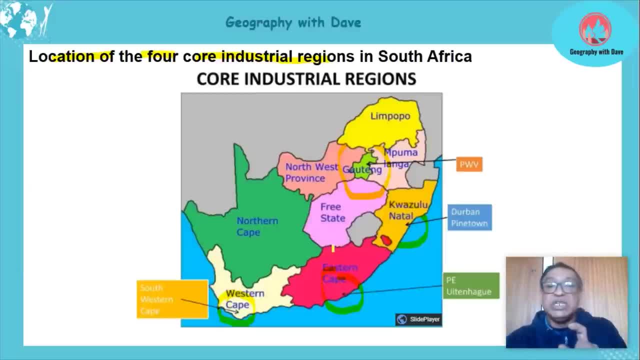 okay. so we basically know the location, all right, and in some cases, the province all right, because howton is making up the pwv area, all right. or in the rest of the cases, the province or the pwva are located northern cape as well, as they say, done business all right. and then, finally, and then the pwv power. next is we were about to target pwv area. we were all thinking about pwc right in the fifth year and we thought, well, why do we need to document that? what is pwv? we use pw Tay to work on db. you, we had to be very familiar with this, which is that they can't be stronger than it either. 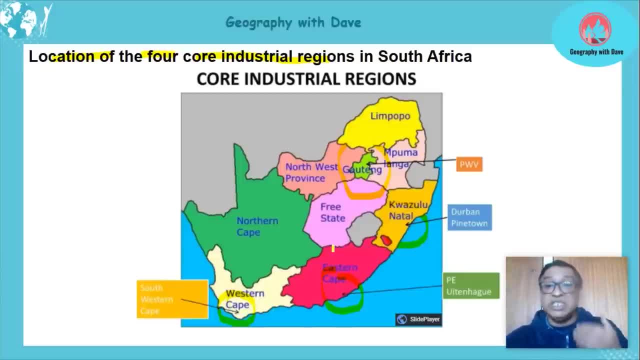 you will, because, because that pwv can eliminate theès most similar to domestic activity of the cases: the province in which it is situated, all right. and another thing to know is that all these three are along the coast, all right, with harbors, etc. some interesting fact? the only one. 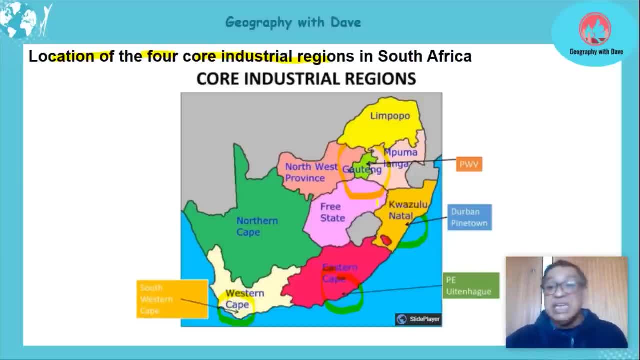 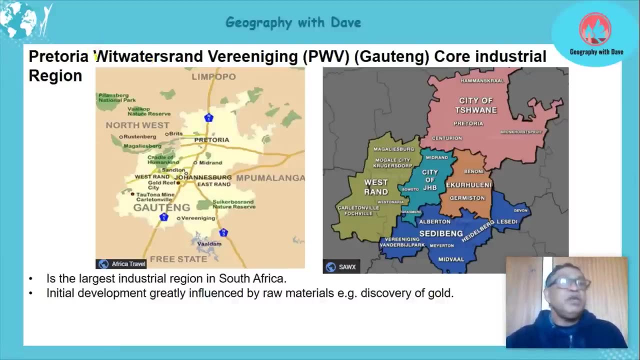 is kauteng, that's more in the central inland that we have from the four of them. okay, now let's start look looking at this. all right now, if we look at the Pretoria Witwatersrand Vereniging, also known in short as PWV, all right, Pretoria, Witwatersrand, and you'll notice I'll be using 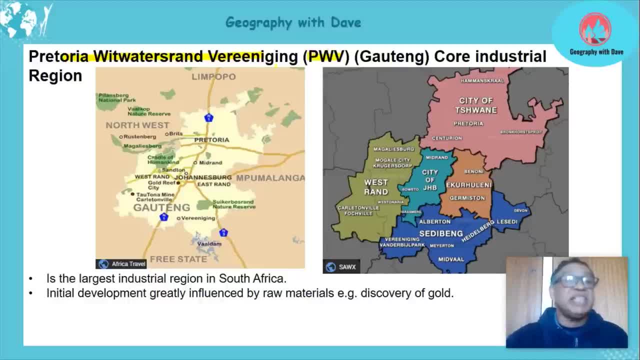 the PWV more often, but you must know that that stands for Pretoria Witwatersrand Vereniging. all right, that stands for, and sometimes it's also called the kauteng core industrial region. so please note the different terminology so that you don't make a mistake. all right, now you can see down here. learners. 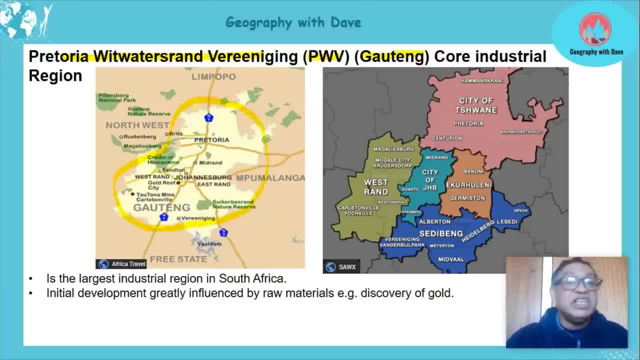 all right, those living in Johannesburg and Pretoria, Etc. would be very familiar with this. all right, I've given you another example here of the different areas. all right, it covers in terms of kauteng itself. can you see Pretoria? all right, and this is the whole Witwatersrand. 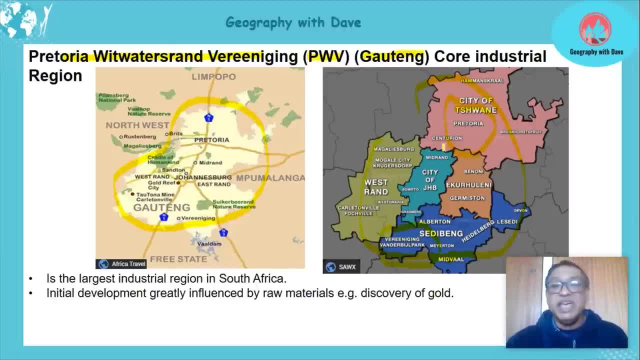 there's Vereniging, all right, in terms of the areas itself, okay, so we can see the area that it covers, the kauteng okay area itself. so one important point: this is the largest industrial region, or core industrial region, in South Africa, the largest, okay, I'll show you more. 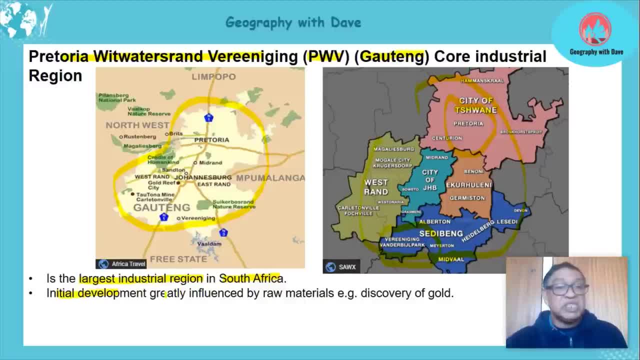 details just now. its initial development was greatly influenced by raw materials. example, the discovery of gold, Etc. this started this off as a mining area and, of course, eventually as minerals came through, you understand the discovery of these different raw materials, Etc. it eventually led to people flocking in and suddenly Industries and tertiary activities. 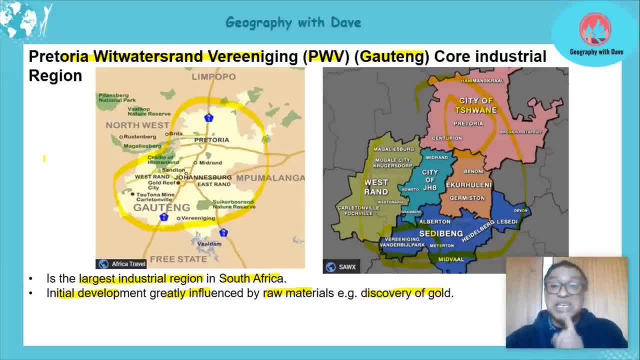 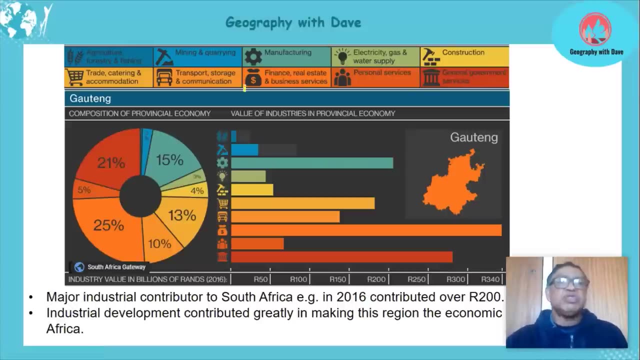 and it's grown so big. but that was the initial thing. just a little background on the pwv area or kauteng area. okay, let's go on right, just to show you something here. I want to emphasize, all right, and I want to move my face before I emphasize, all right, uh, I want to, and, of course, this note: 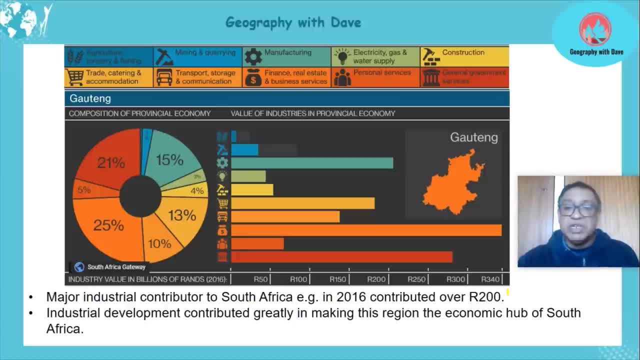 is missing something here, okay, which I want to put in. I don't know where it disappeared too. I want to write the word million here, okay, all right, million, and my writing is getting better. okay, right now I want to show you something here in terms of its contribution. okay, now we look at this in billion rather, and to apologize, 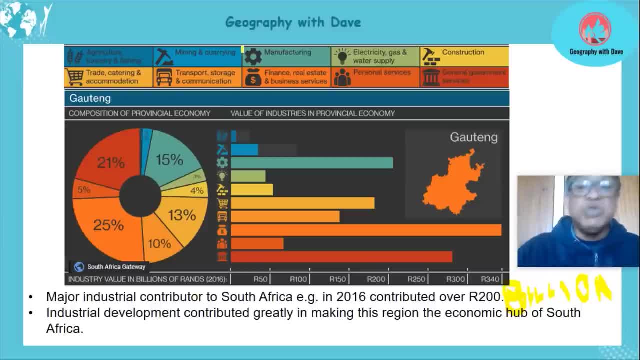 in billion, not million billion. and I want to show you something here. all right, manufacturing, manufacturing- all right, okay. and if I look at this same one, that color there's it here- and if I go down, okay, I can see that manufacturing in this area, okay, contributed 200 billion in 2016.. can you see the massive amount that it's contributed to? it's huge, you. 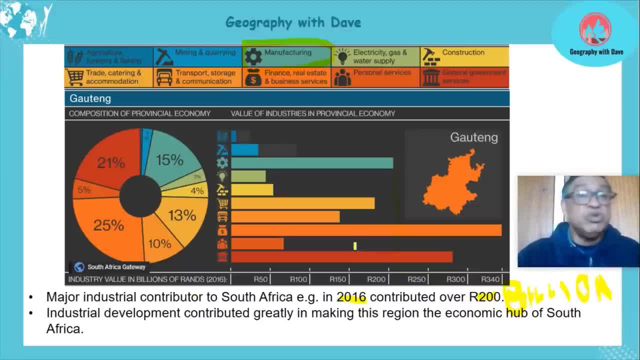 understand it's huge in terms of its contribution. okay, and, of course, looking at this, it's 15 percent. okay, massive in terms of this. okay, this region, so we can see it- is a major industrial contributor to South Africa and I do apologize, but you can see my billion day, okay, right, so it's. 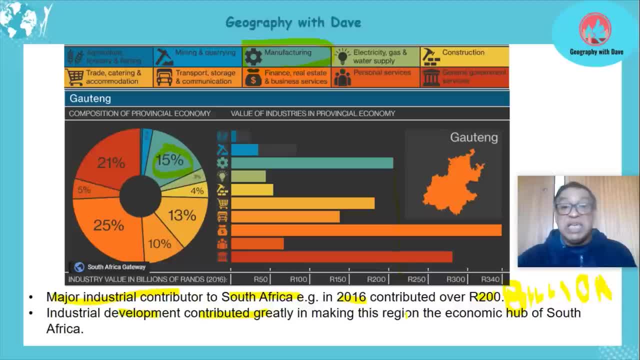 industrial development contributed greatly to making this region the economic hub of South Africa. it's where things happen. you know, when you find you visit your family, if you're living in housing and you go in the outlying areas where people are not, uh, employed, Etc. one of the questions I asked you where? oh, you're from Johannesburg. how, how's the? 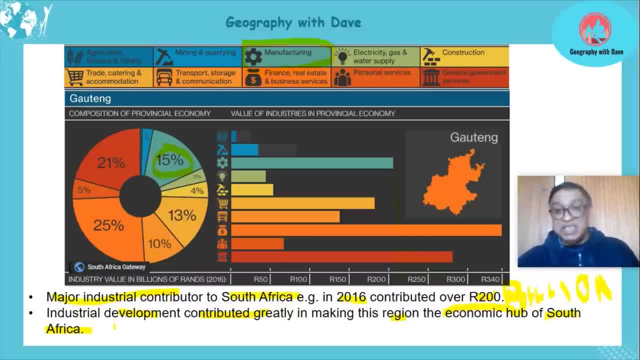 job is there in job, but we hear there's a lot. actually there is an unemployment problem, but everybody sees it as the big industrial area of South Africa, which, it is all right, economic hub and it's one of the big centers of industrial development in Africa on its own, you understand. 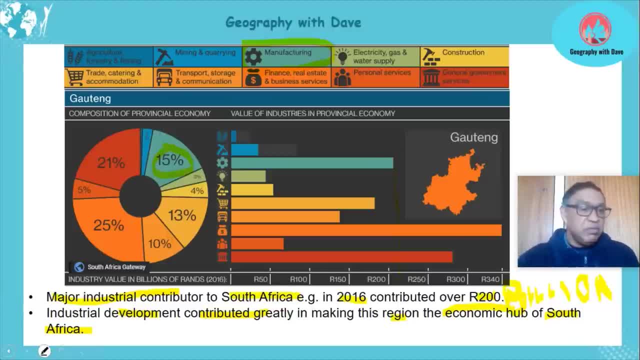 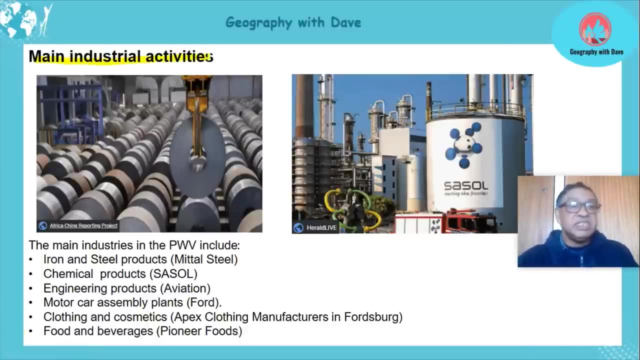 if you, if you look at it. okay, so it's huge contributions all over to the economy and, of course, many issues related to that like infrastructure, Etc. okay, right, main industrial activities. yeah, the main industrial activities in the pwv- learners, please note I am using pwv now, which represents Pretoria, which represents how thing? all right, iron and steel. 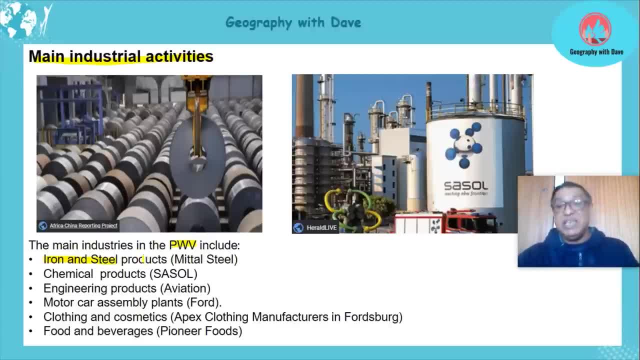 products is huge in this area- and, of course, Industries linked to the iron and steel- okay, production of vehicles and kitchen utensils- I can go long on, all right- and one of them is the big company as metal steel. okay, that's in this area, all right, that is one of the big ones. 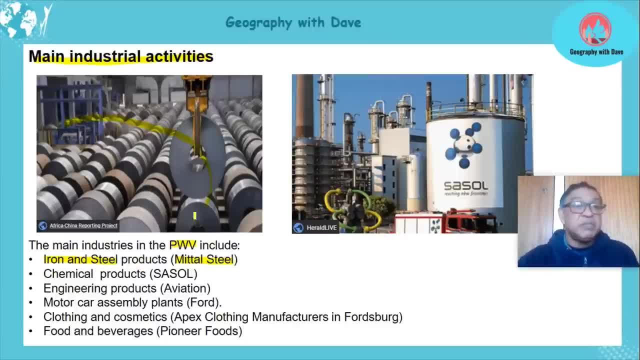 and another thing: beautiful. can you see the steel being produced here, by the way? okay, and then the chemical products. there's so many different chemical products. I'm using Cecil, okay, that takes the coal and makes fuel. okay, which supplies a lot of the fuel, or significant amount of fuel, to the 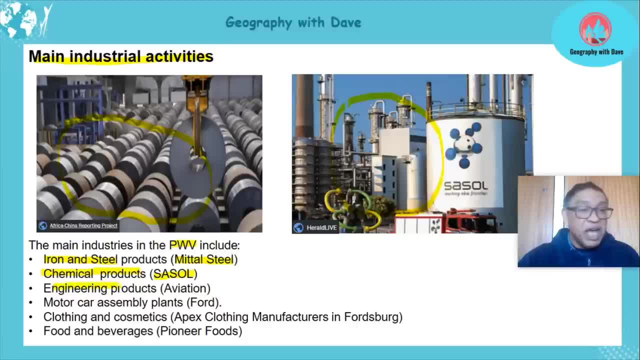 country also. okay, engineering products, example for aviation, involved in parts of aircrafts, Etc. motor Ford is found here. you understand Ford. okay, these are some of the big ones, doesn't mean they don't have other Industries. learners, I'm giving you some of them that are huge in this area: clothing and 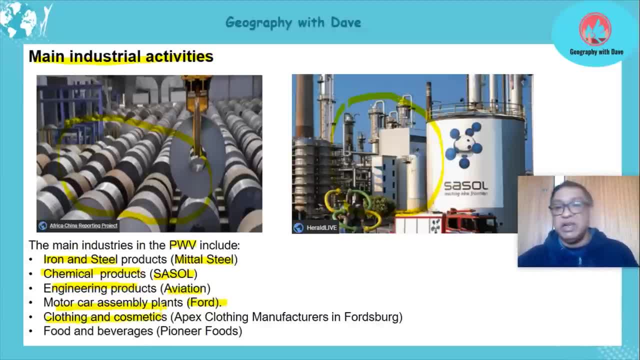 cosmetics. I know learners, you like the clothing and cosmetics, but anyway, you'll get a good supply in this area, like Apex clothing manufacturers in Fortsburg. okay, all right, so they have lots of clothing manufacturers. food and beverages also in this area. that's huge- like Pioneer Foods where you'd get one. just examples. 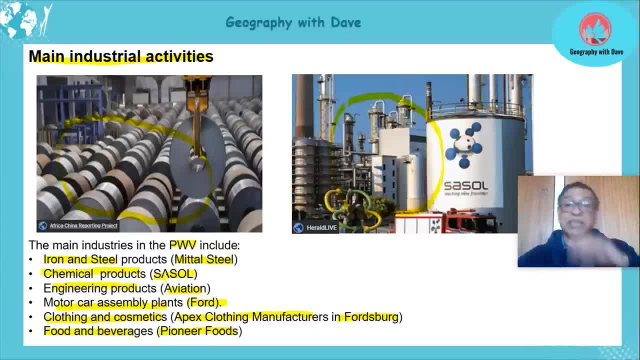 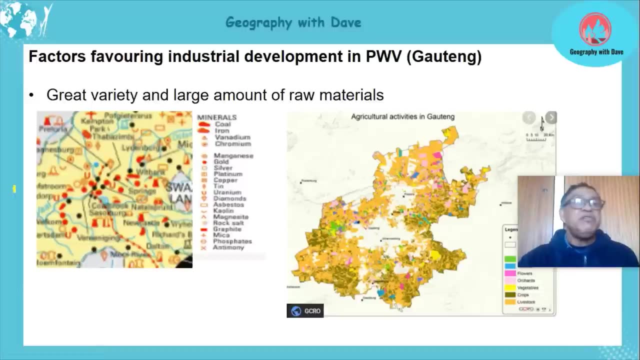 that are giving you. there are other companies also. I just gave you an example- that if you're driving around, you may see this and say, hey, there's food and beverages being produced in this country, or or rather in hauting. okay then, why is this area popular in terms of industrial activities? so we look at factors favoring industrial development in. 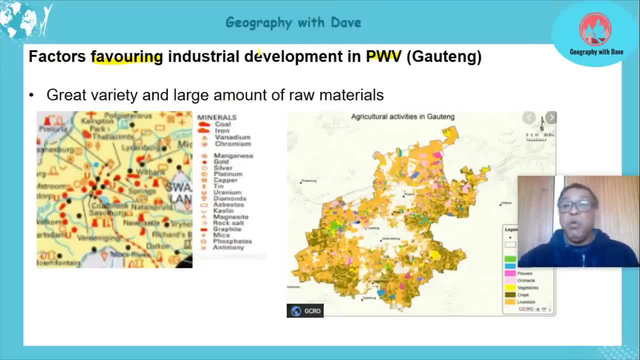 the PW all right regional housing region. one strong, strong point that we will look at is the variety and large amount of raw materials. now, if I look at this coal, iron vanadium and the symbols, and if I look at the housing region here, it's full of those symbols, massive amount of symbols telling you that the mining raw materials 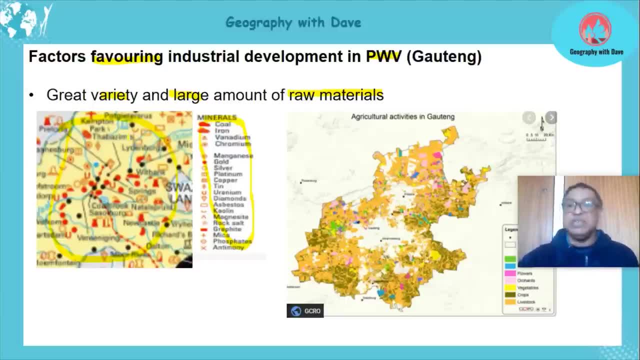 of raw materials from mining is huge in this area. what a boost for uh Industries in this area. you got your iron and steel, or iron ore, rather right near you to produce iron and steel, and how many products are made from iron and steel is unbelievable and it's bulky learners. to transport them is massive. okay, it's expensive, so you need to. 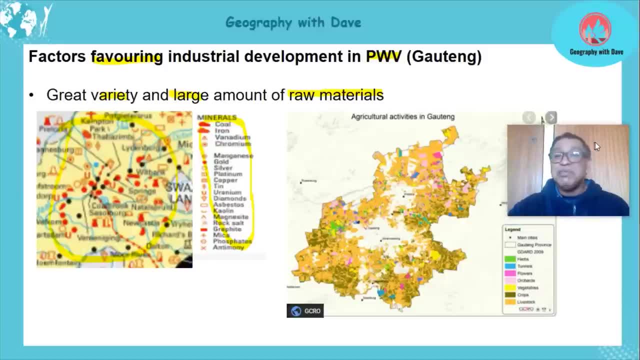 have it near you now it's not all. remember, mining raw materials are one thing, but we also look at agricultural raw materials. okay, that come through, and this area has also got an abundance. look at all these things: herbs, orchards, vegetables, talk. all right, that's used in manufacturing. in the lesson on the manufacturing and agriculture and 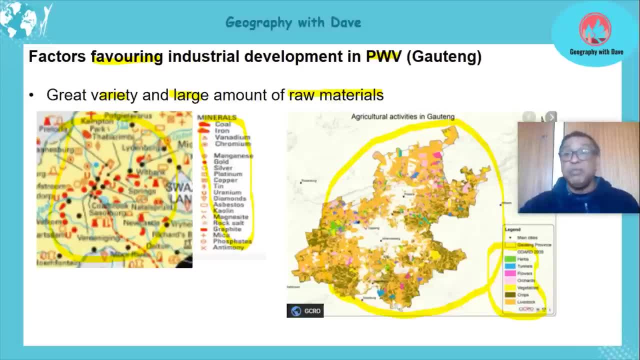 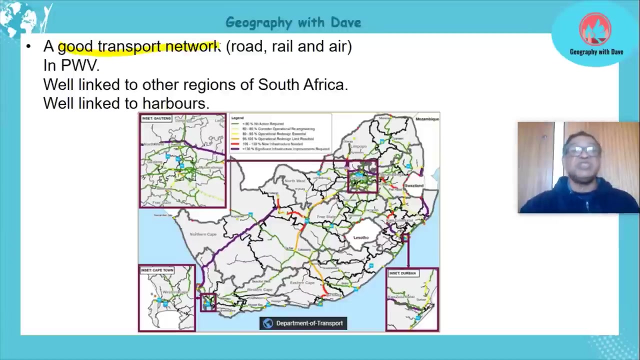 the contributions, you notice that even these raw materials, all right, produce a lot of things and encourage Industrial Development in those areas. okay, so it's raw materials, no problem in housing, whether it's coming from agriculture or whether it's coming from mining. okay, the next point: a good Transport Network, in fact an efficient Transport Network, whether it's road. 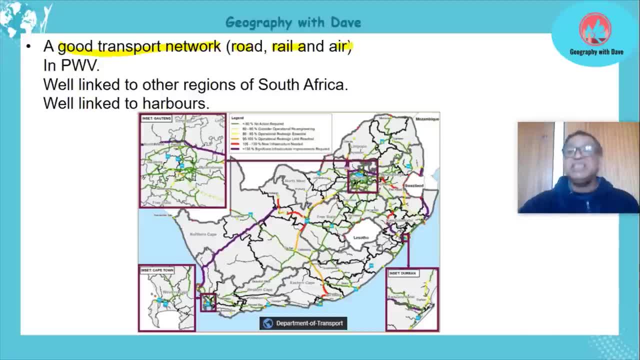 rail air. there is enough Transport, okay in the PWV. okay, that's one thing, all right, plus another: positive factors. learners, you must know that we can't just look at the PWV as such and say, excellent, because the PWV wants to sell to other areas, okay, so it's well. 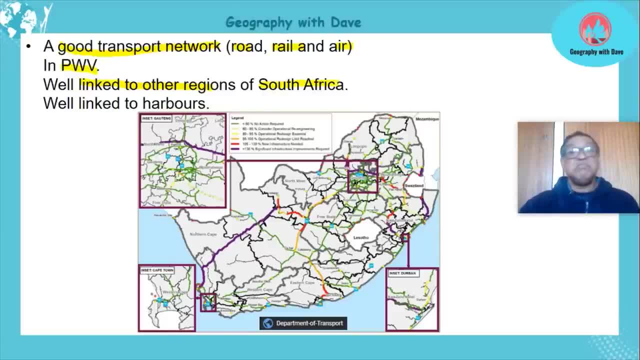 linked to other regions in South Africa. okay, I've got this little sketch here: PWV- can you see it? look at the networks whether it's roll rail all to all parts of the country. so this well-developed transport Network allows us to transport stuff from the PWV region to all areas. okay, which is brilliant for the PWV region all. 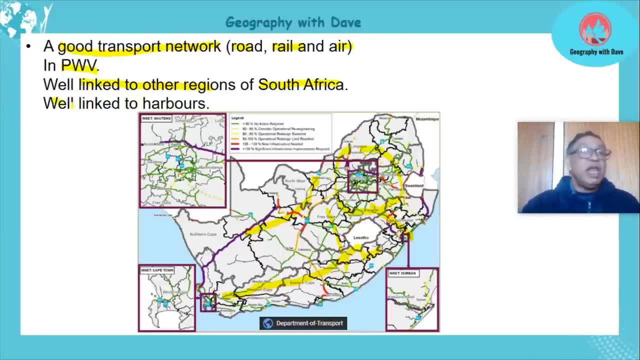 right, and another thing that we need me to look at: the well linked to the harbors. all the harbors are found in these regions and you notice the transport networks are efficient when it leads to the harbors, because you must remember how they can't transport. 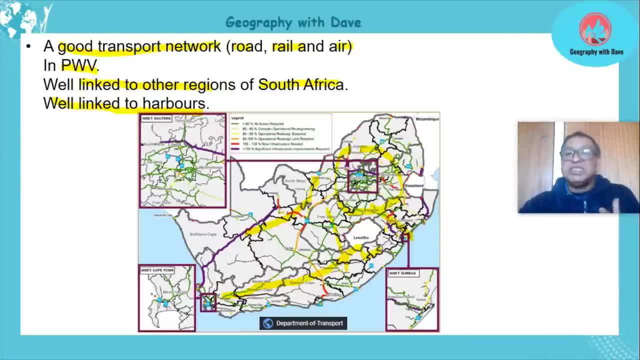 steel in aeroplanes either can, but it's ridiculous. the costs are way, way out of the range. you understand, it's not even worth doing it. so it has to be transported, you understand, via ship, through the harbors. so we're well linked with that also. okay, let's go on large market, okay, the. 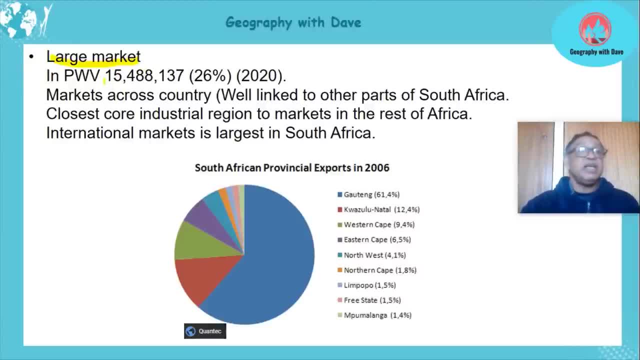 should be saying more. the Khouteng region, right, the Khouteng region. I'm going to put a G here. in this area, the G representing right has 15 million 488 137- well, I can read my figures- which makes up 26 percent of the population. this step was taken. media between 2020. Okay, so it's massive. 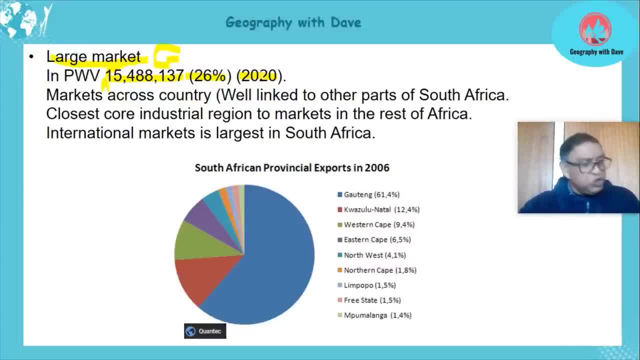 So the immediate market learners. we're producing in Gauteng and once again, I promise you this is only water. all right, we're producing in Gauteng and we have a market around us that can buy our goods. How much are we saving on transport costs? 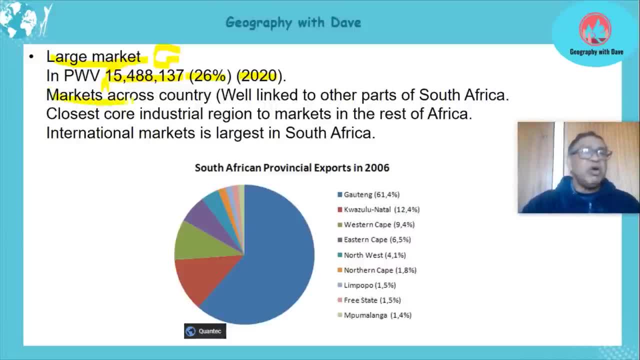 Brilliant, All right. And we have markets across the country, across the country, You understand, And this well-linked transport routes help us transport. So we have markets across, all right, And remember it's the closest core region to markets to the rest of Africa. 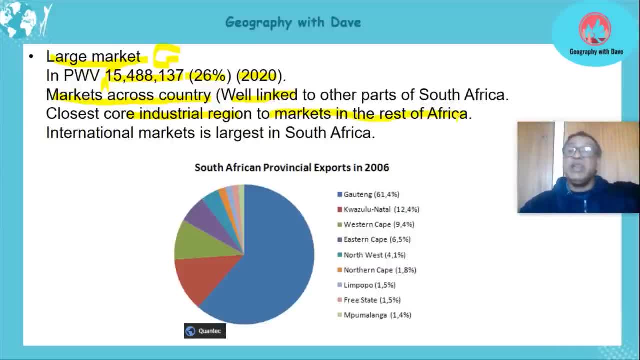 It's right on top, Okay. So if we have to use rail or whatever to transport things to the rest of Africa, we are the, or rather the Gauteng region. okay, is the closest to the rest of Africa, which also is a positive. 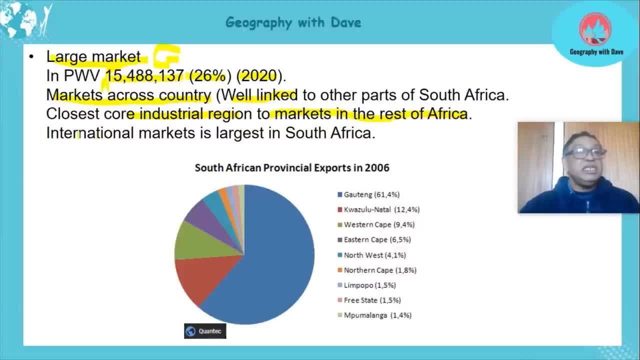 Right. Okay, In terms of that, all right. international markets: largest in South Africa. Okay, Look at this. provincial exports in 2006.. Okay, I found this little thing. It may have changed a bit, but as I always say, guys, learners that you have to look. 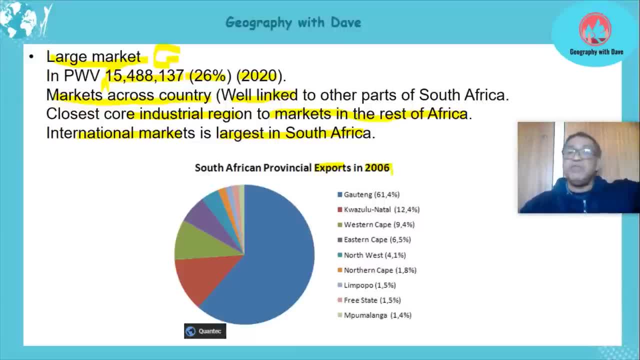 at the resource that's given to you. So maybe your examiner will give you for 2014 or 2020.. We never know. use that, But Gauteng is- look at this figure- 61.4% compared to anyone else. 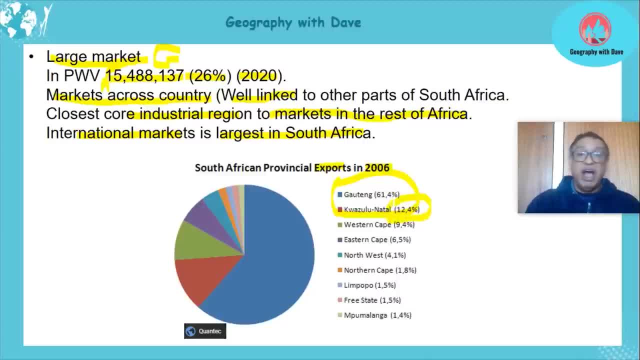 And then you go to Gauteng, to KwaZulu-Natal, which is 12.4%, massive difference between these two areas in terms of contribution with exports. Okay, So can you see how big this Gauteng Pida is. 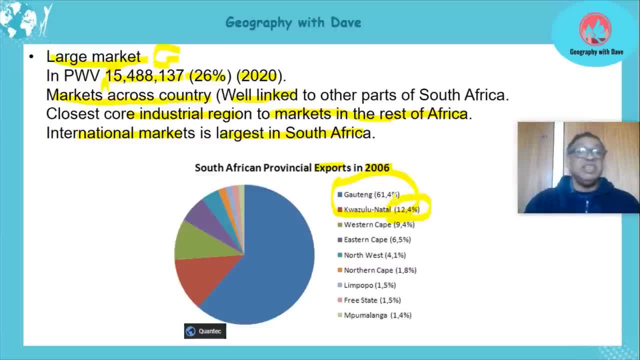 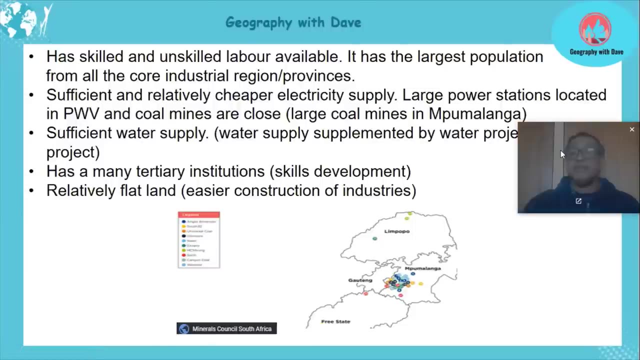 There's a very big difference. Okay, pwv region is massive, okay, so a large market is available, all right, because it can export to so many places. so it definitely will encourage, uh, industrial development in this area. okay, now we, this area, has skilled and unskilled labor available. okay, all right. and we must remember: 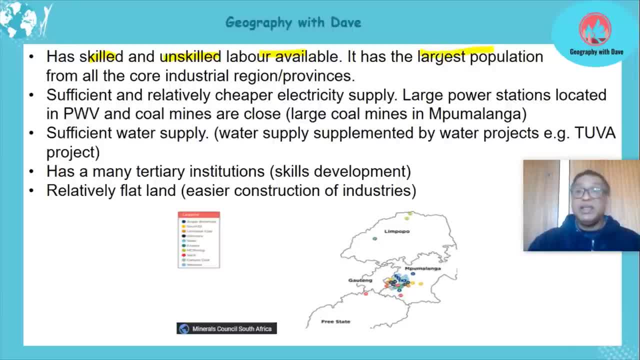 it has the largest population from all right. all right, so skilled and unskilled labor is available right there with so many million people. all right, you've got enough labor available in your area. okay, of course it's not saying that there's specific skills. that would happen, it happens. 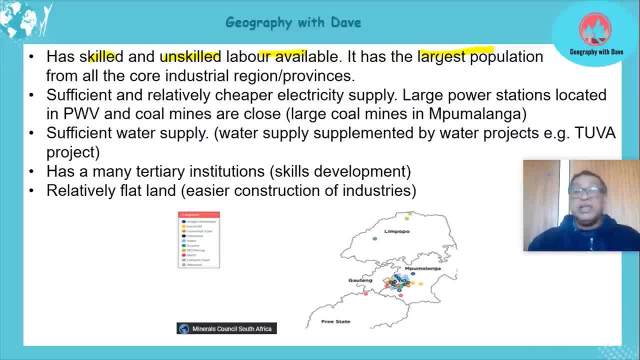 everywhere that may require somebody from the outside, that does happen. hey, right, sufficient and relatively cheap. i'm using the word relatively cheap, hey, remember, compared to other regions we'll talk about later electricity supply. okay, relatively cheap. why we look at it. large power stations are located in the pwv. 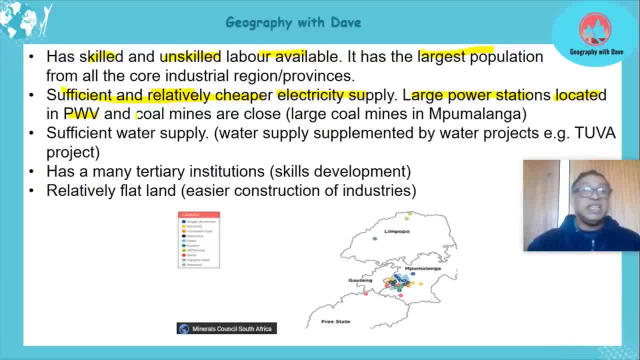 and what makes it possible- yeah, learners, is that the coal mines are close. all right, coal mines are close, large scale, large coal mines in impumalanga. look at here, guys, there's gouting there. can you see how to? and look at this area, showing you different coal mines here. 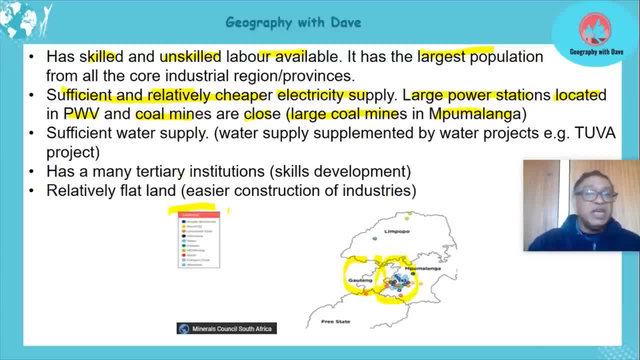 all right, right there there's all the different names of- we don't need to know names, etc. but i'm trying to show you visuals in terms how close. so to produce electricity in this area is not a problem. and then sufficient water supply, and again you may question what. 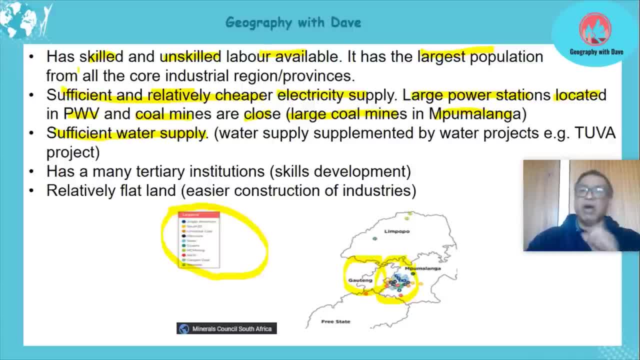 you understand? uh, how can it be? yes, there are water problems, but there were initiatives put in place, learners- to actually try to overcome these challenges. example, uh: water supply supplemented by water projects like the tuva project, falchugela project, where water was pumped from the kwazulu natal area into the khauteng region. so we have supplemented our water. 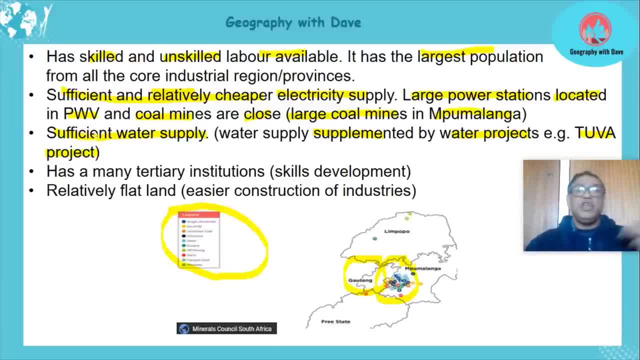 okay, there can be cases where you may find that droughts occur, and that happens. yes, these are issues, but we have sufficient water supply. I want to go into this whole tuva project. you've done it in your other grades. eh, I know this may seem like not such a significant factor to the 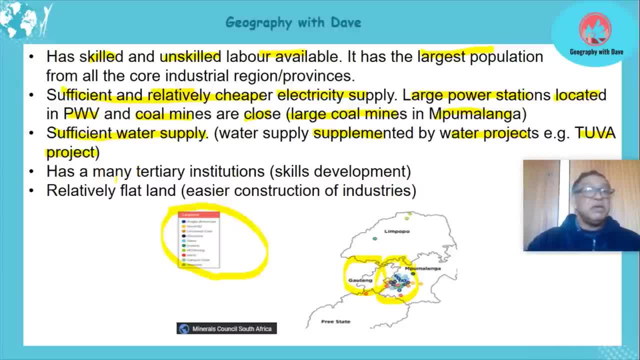 rest all right, but it's a contribution nevertheless. many tertiary institutions in the khauteng region, many universities, technicons, technical colleges, so skills development, learners, shouldn't be such an issue. there are issues where population is growing and there's not much space which needs to improve, but there are a lot of institutions. all right, relatively flat land. 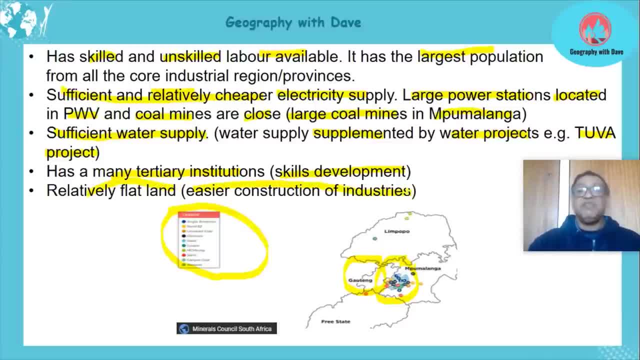 okay, it's easier for the construction of Industries and movement of stuff Etc. okay, I said relatively flat. not every area is flattened counting. so if you come to counting and you see a hilly area, don't say Mr Dave was wrong. there are areas that are healing. but of course when you answering go with. 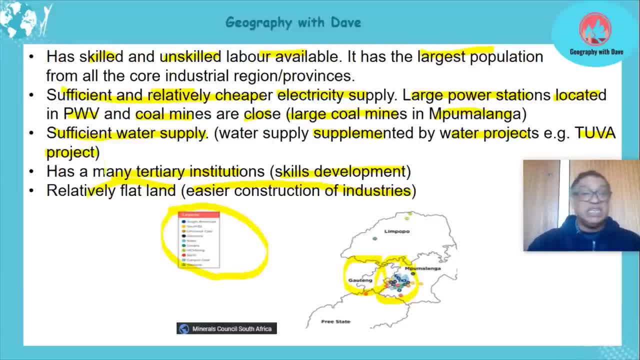 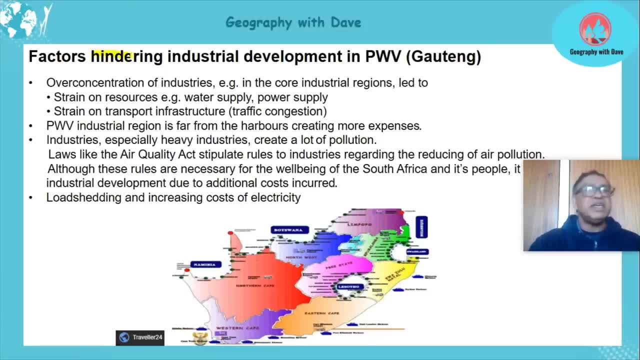 the main factors. first, you understand, like raw materials, Etc. okay, let's go on. factors hindering that work against industrial development in the PWV counting region. okay, so over concentration of Industries. I know we're repeating this. we've done this as factors favoring and hindering, but now we're being specific to the areas. right, okay, led to the strain. 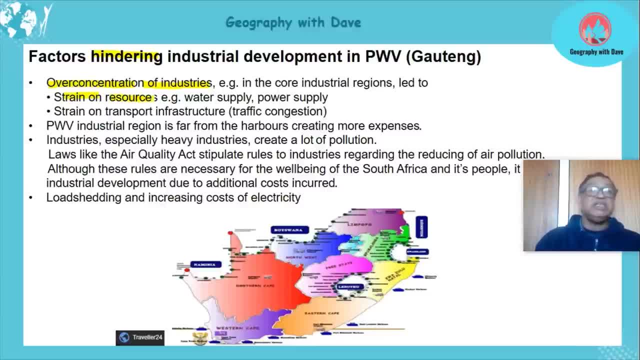 on resources: okay, too many Industries in one place. water supply, power supply: it's straining it. okay, because there's such a large amount of it here. strain on transport infrastructure: traffic congestion: okay, it's a hindering factor because to send your goods out from the PWV region. 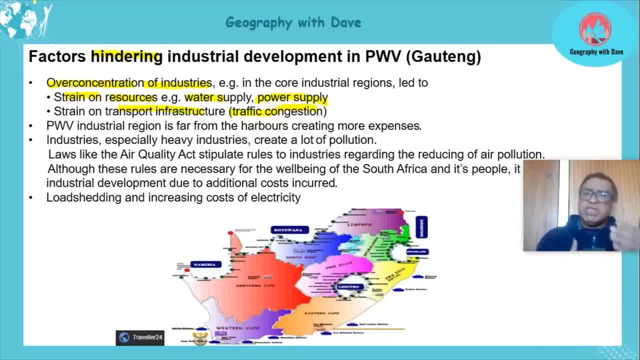 okay is a problem. okay, because sometimes you get traffic jams, your goods are not going out or the raw materials are not coming in. these are massive problems that we experience. okay, PWV industrial region is far from the harbors, creating more expenses. now, learners, yes, there is a. 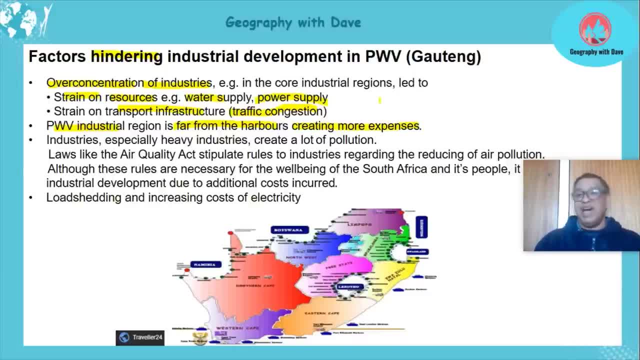 developed a transport network leading to the harbors, like Durban etc. okay, but still, if you look at it here, all right, counting okay in those regions, and then you have to move it to the harbors, each Arbor. you see there has to be a distance. don't look at the map. distance look. 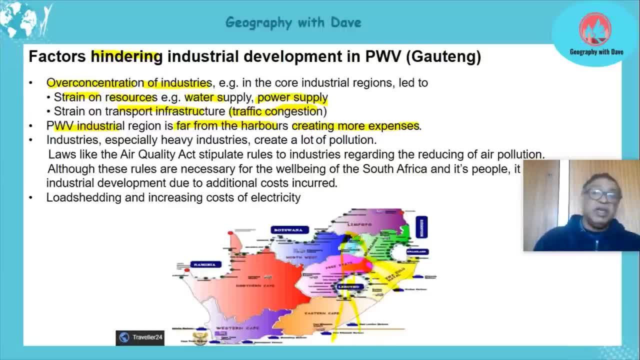 at the real distance. eh, all right, it's a real distance, like from from counting depends where you are: approximately 600 kilometers to the Durban Harbor, which is a huge distance and it's costly. okay, so that's a different one. also, industries, especially heavy Industries, create 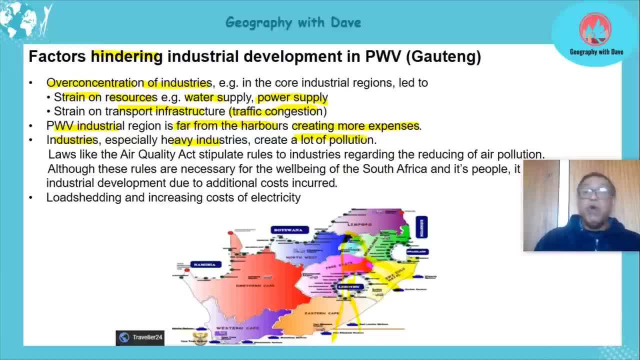 a lot of pollution. okay, on its own, pollution is a problem, but of course, governments want to bring in laws like air quality act with uh, rules for Industries regarding reducing of air pollution. all right, reducing of air pollution, so what actually happens here? all right, it's good, these rules, this has been. 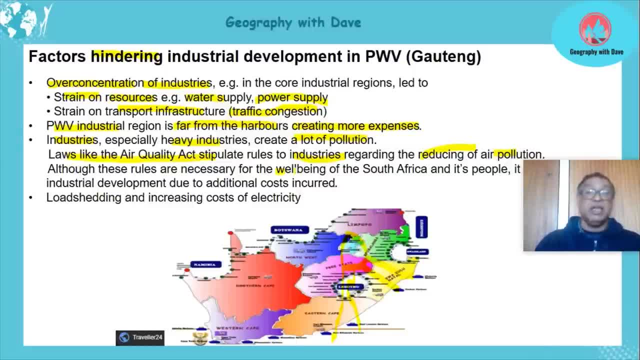 explained before, but I know I need to bring it into context of how it's good for the well-being of the people and, okay, let me move my face a bit. all right for the people of South Africa and the well-being of South Africa, but it may hinder, okay, uh, industrial develop due to additional cost to 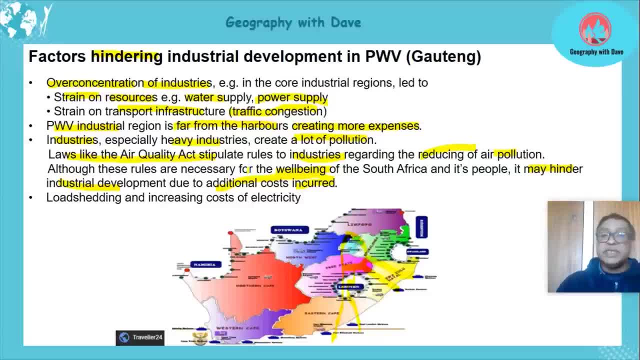 put this in place and Industries may move somewhere else in the country where the laws are less stricter, or to other countries, you understand, uh, where it's easier for them to put in there and and pollute, especially multi-corporations, Etc. okay, so it may pull industrial development if more laws are. 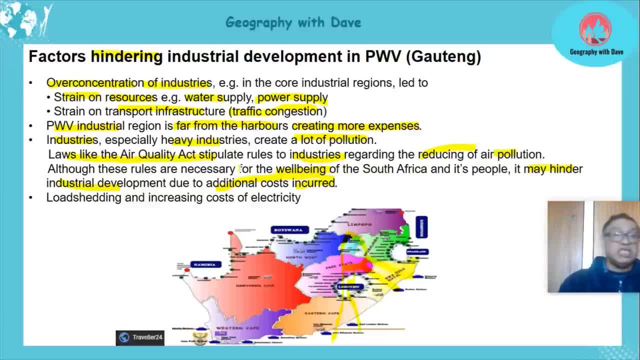 implemented and strongly implemented, and South Africa is trying to cut down on the environmental damage. okay, load shedding and increased costs of electricity. unfortunately, it's a reality. eh, uh, load shedding: there is enough, or should be, sufficient power supply with the resources we have. okay, but unfortunately, various. 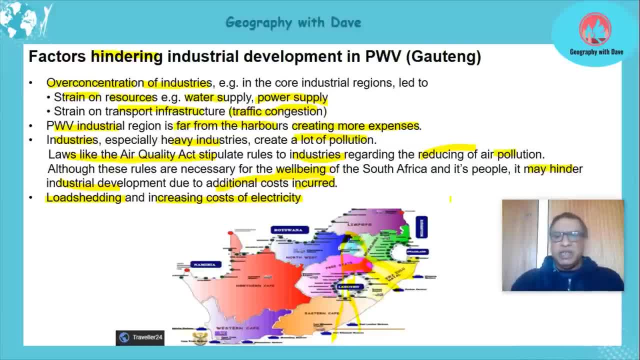 factors I've mentioned over my lessons. you understand old infrastructure, uh, the sort of corruption issues, Etc. and we all- government does- sort that out so that we can get on with providing enough electricity for all of us, not only for the Industries. eh, for us learners, we don't want to be in. 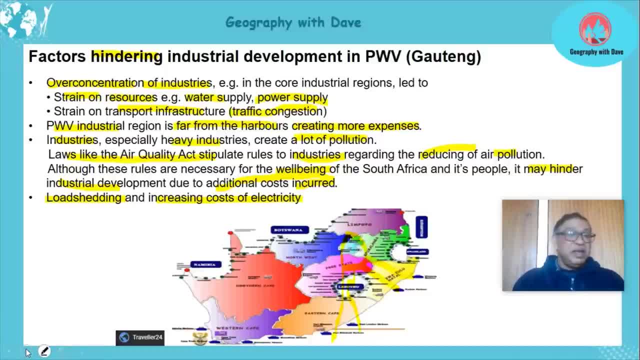 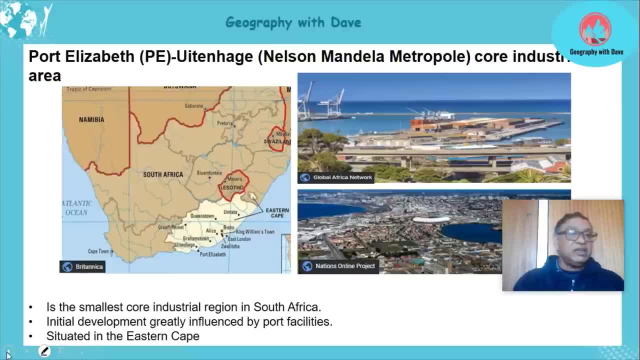 the dark all the time. eh, all right, let's go on. and I'm not going on, all right, and I need to get back to the other slide and I don't know why it's not coming in. and there we are. okay, Port Elizabeth, PE in short for Port Elizabeth, eutonite all right, also known as the Nelson Mandela. 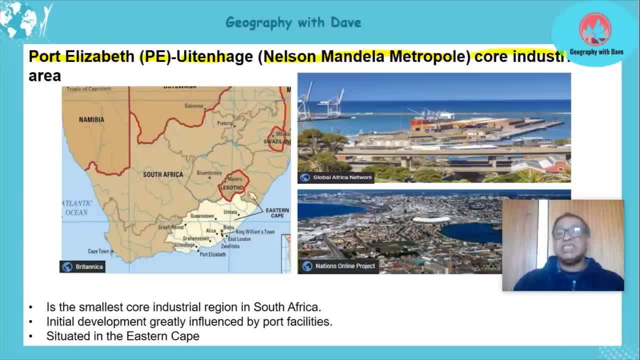 metropole core industrial area. okay, and my mouse is taking a bit of a jump. okay, first of all, we know it's in the Eastern Cape and it's there we are. that's where the eutonic, or Port Elizabeth eutonic core industrial areas. you can see the major Harbor. eh, that's there. 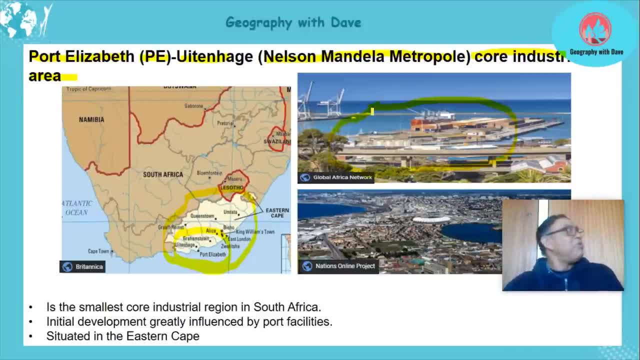 already you can work out to a certain extent, learners, how it's going to Advantage the area. it's already because you guys are brilliant, you understand. maybe I don't have to teach the rest of this lesson. okay, you know already. okay, you can see another view of Port Elizabeth around. 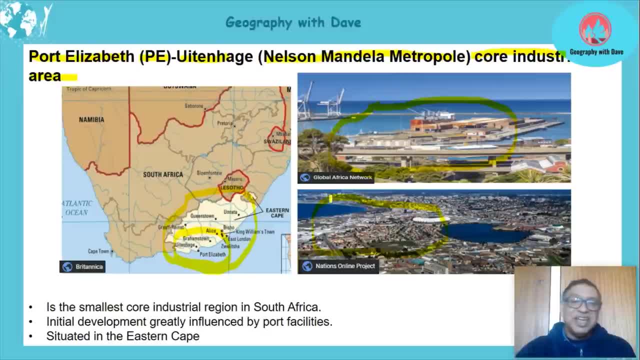 the Harbor and the ocean, Etc. okay, that's it. and of course, your leg is not far from there. this whole region is covered there. okay, now let's look at some facts. it's the smallest core industrial region of in South Africa. now, please learners. I said smallest. 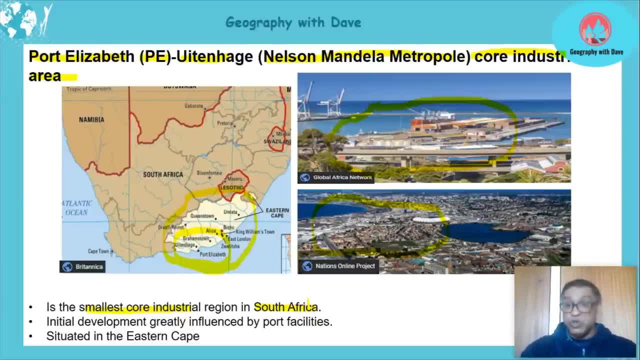 I didn't say insignificant, its contribution is huge. also, you understand. okay, it's only four core areas, so its contribution is used. so please do not get the wrong impression right. and the initial development greatly influenced by the port facilities. obviously, if you've got a port there, Industries want to be there. cheaper costs of importing certain. 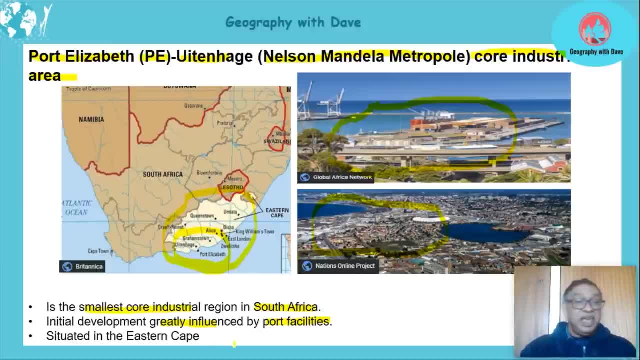 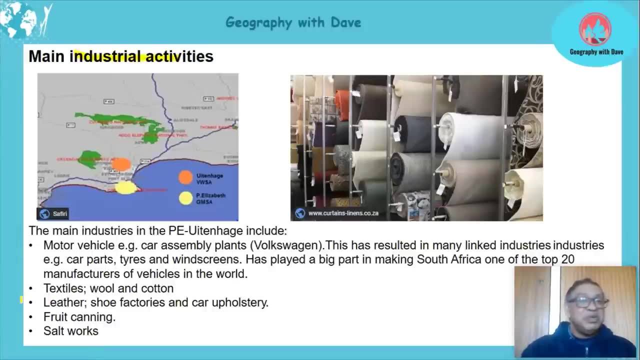 things they need and exporting. okay, and of course I mentioned it's situated in the Eastern Cape. okay, right, let's go on. learners, our main industrial activities. okay, we see here. it includes motor vehicle car assembly, right, and of course this has resulted in many linked industry issues here. okay, like car parts, tires, windscreens- okay, all is needed. and if the car Industry is, 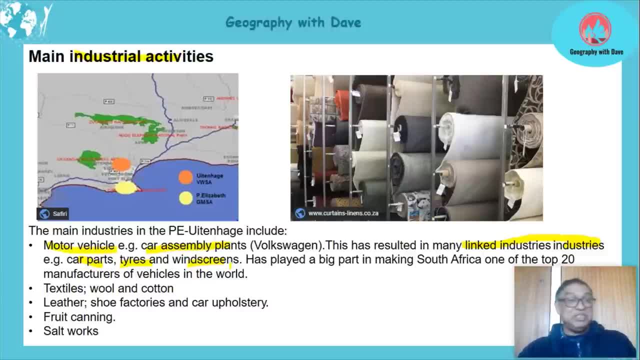 there. okay, why not? something you damage? you already got the. you need tires, whatever. it's coming through okay and it has played a big part in South Africa. uh, South Africa is one of the top 20 manufacturers of vehicles in the world. in many in years it was remoted. i know it's shocking, right, this statistic? all right in the. 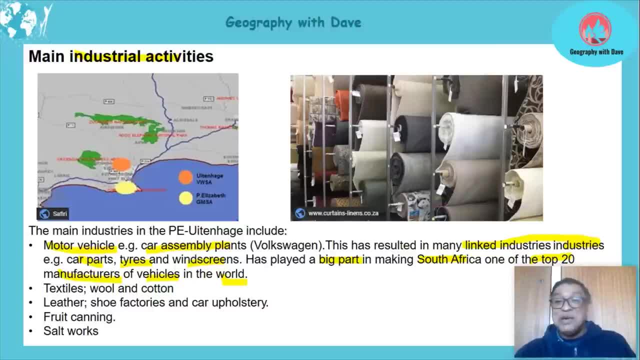 earlier 2000s it was number 18. okay, we don't know this sometimes, eh, but it's huge and the p, the port, elizabeth, euton egg area, played a huge part in this right. others is textile and cotton, leather and shoe factories. okay, up, car upholstery, fruit canning and salt works. now, obviously you can. 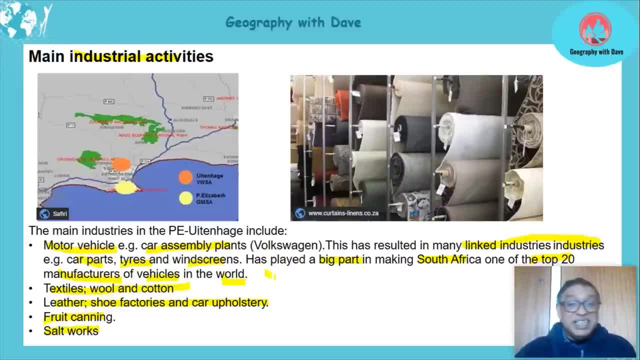 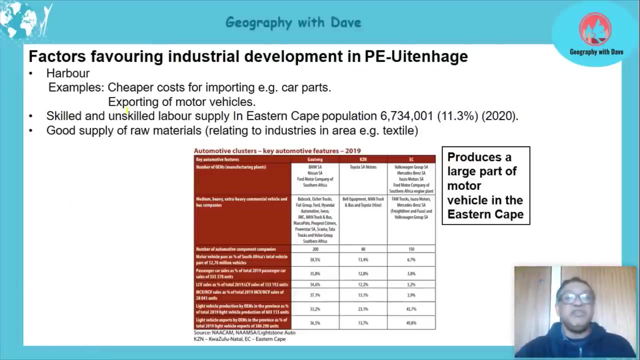 see, these are other industries and these industries- learners- have obviously been influenced by the raw materials available in the area. remember, raw materials play a big part also in determining what sort of industry you will have in an area. okay, let's look at factors favoring and obviously you would look at. 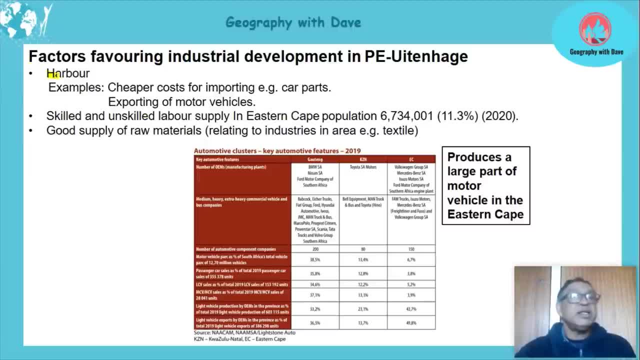 the harbor: okay, the harbor massive factor, okay, massive cheaper costs for importing, example, car parts: okay, because it comes through ship much cheaper. and exporting of motor vehicles: all right, huge, all right. of course there is skilled and unskilled labor available: okay, eastern cape has a population of six million seven hundred and thirty four thousand and one ah. 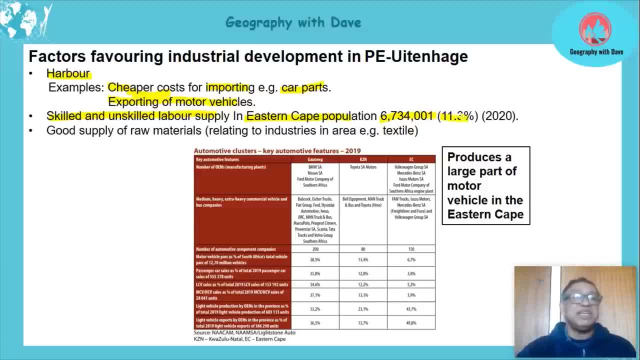 the one also is included: eleven point three percent. eh so, remember i'm talking eastern cape, all right, uh, of course, this core region will influence a larger part around the eastern cape. okay, in terms of labor supply. okay, please note it's eastern cape and not just the peuton area, but there's a large area. 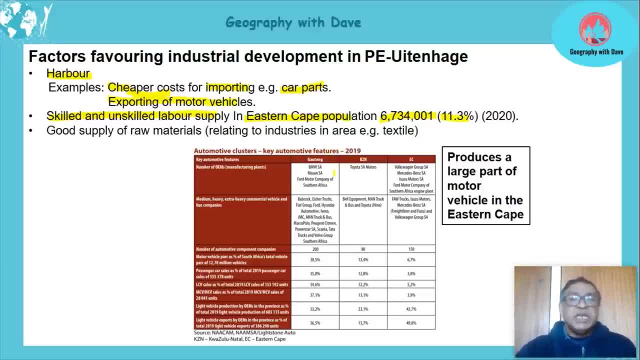 available, all right. uh, now, if you look at this little thing, okay, look at here, all right, the different cars that's produced by the eastern cape. okay, and we look at the number of, uh, automobile component companies. look at this high. all right for a smaller region, all right. motor. 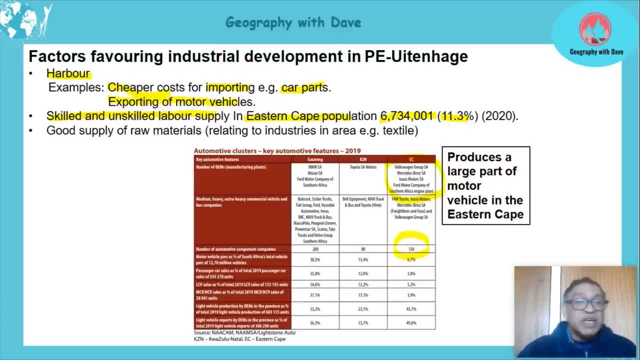 vehicle uh percentage of south africa's total vehicle power uh pack of of 27- 12- 12.79 million vehicles: 6.7 percent, can you see it? and if you look at light vehicle production, 43 percent, can you see it? these huge things. as long as you don't have to know these figures, all right, as i said, you'll. 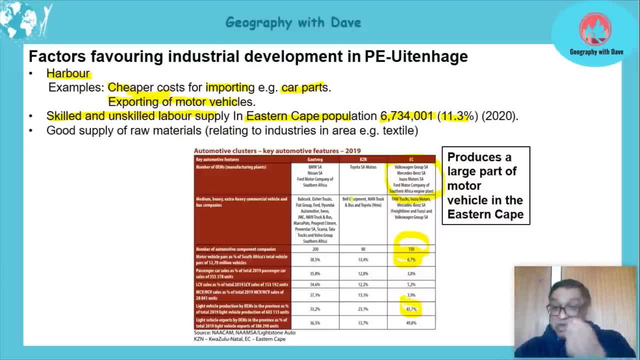 get a resource with actual figures, which may be different from this. okay so, but just giving you an idea of the significance of this motor car industry. okay, that's found in the peuton area. now, i know this is the eastern cape. uh, it produces a large amount of parts in the eastern cape. 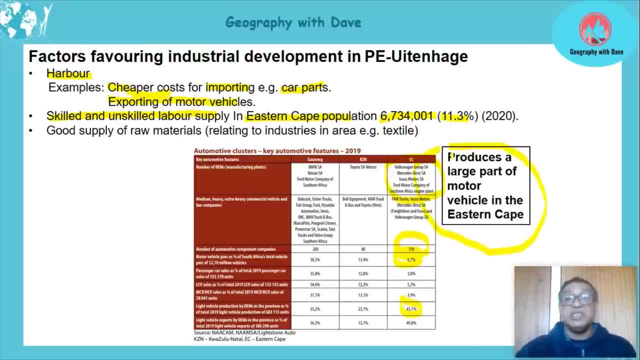 okay, produce a large part of motor vehicles in the eastern cape. when i say produces, i'm referring to the port elizabeth. so, yes, the port elizabeth may not have this. uh, eutonic may not have this figure, but a significant amount of this figure is found in the pe eutonic area. so this figure. 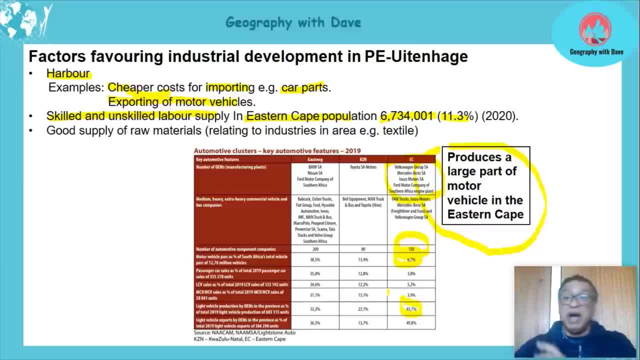 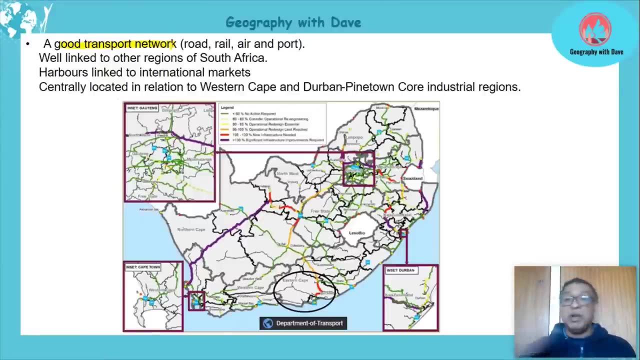 is for the eastern cape, but, of course, a significant part coming from the pe eutonic area. okay, it's massive, massive letters. okay, right, a good transport network. i know parts of the eastern cape are not well, uh, sort of developed in terms of infrastructure. i'm putting the focus on the 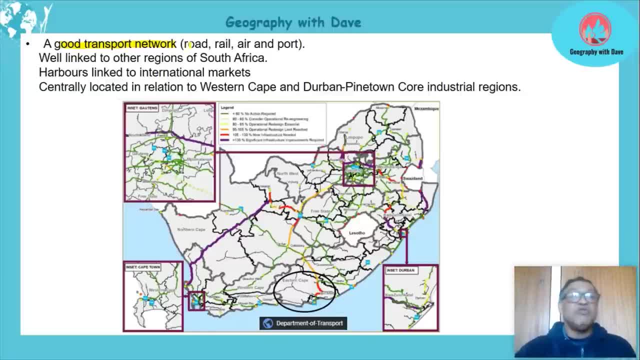 pe eutonic area. okay, so don't confuse it, it's road, rail, airport. we have all these things in this area. okay, more emphasis on the port, the harbor. it's well linked to other regions of south africa, as you can see here: massive networks, harbors linked to international markets and for importing. brilliant, all right, centrally located. 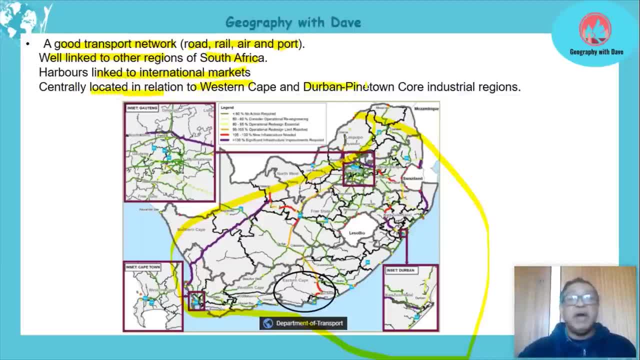 in relation to the western cape and durban pine town. we can even go provinces there. we are here eastern cape and there's durban pine town, all right, and we have the western cape here. okay, maybe slightly towards the western cape, but it's quite simply located. we have two markets nearby. okay, two markets nearby. 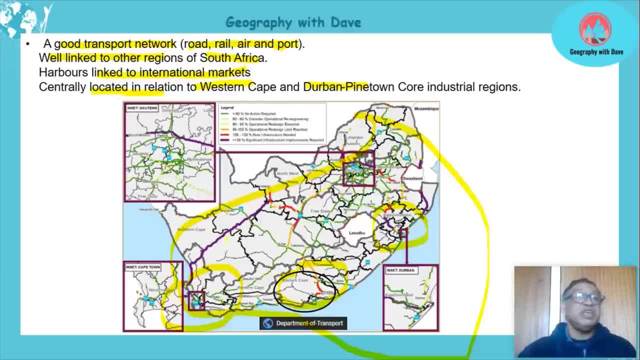 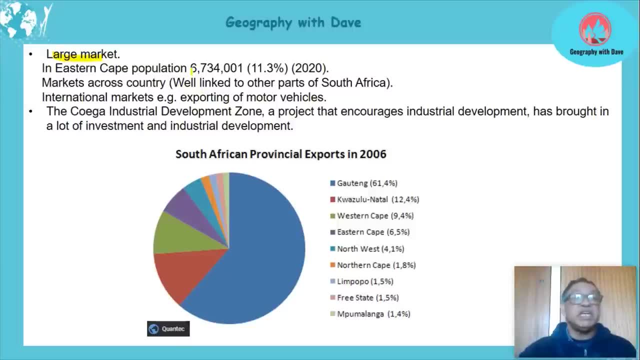 can you see that? brilliant for that. and of course, the infrastructure, large market. of course the eastern cape population- i told you already, over six million, 11.3 percent. there's a market there. markets across country also because it's well linked to other parts. international markets through the harbor, which also allows for exporting. 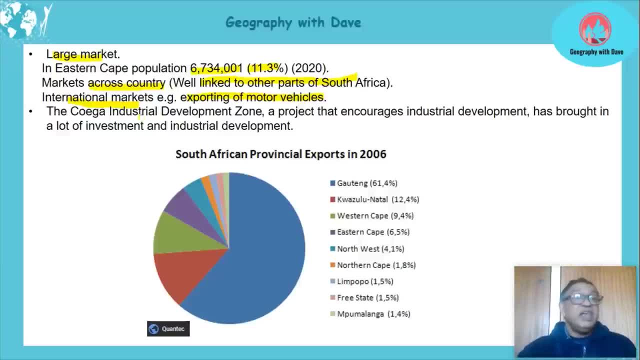 of motor vehicles, etcetera. okay, and then a last point. you don't have to really know the kutha industrial development project, but it also played a huge part. this k alcanzed school industrial development project- actually, what is it? it's a largeэ project, not the full definition learners, but the project encourages industrial development. 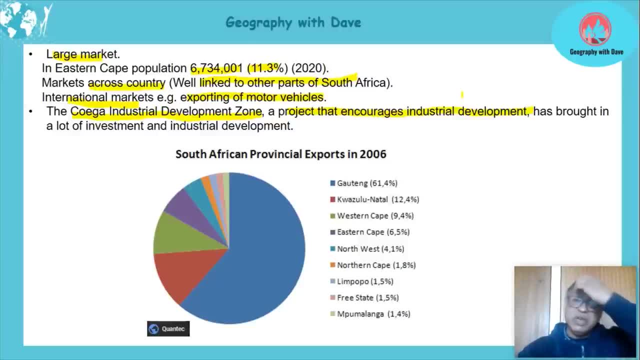 in areas. it's initiatives that put in place to encourage more industries, etc. we're not going to go into detail now. in a later lesson we'll deal with specific industrial development zones etc. but you just need to know that it encourages industrial development. okay, and kuka is about. 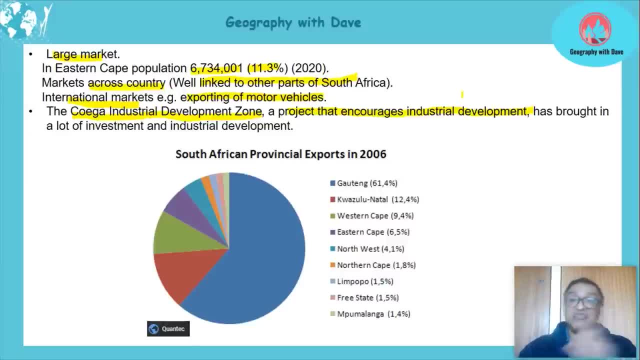 the largest industrial development zone in the country. so what has this done for this area? it's brought in a lot of investment, learners and industrial development. okay, it's grown. it's grown all right in terms of because this uh industrial kuka industrial development zone is in this area also is affected and favored. you understand it's a factor that favored this area. 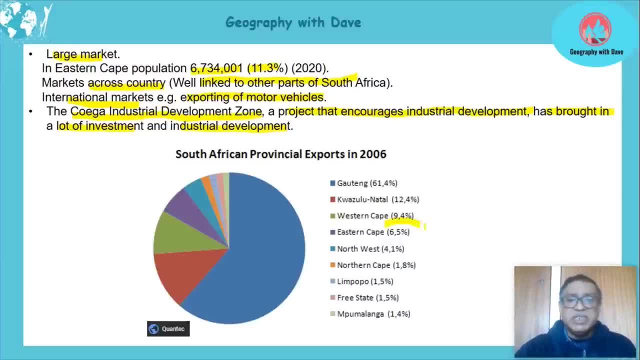 all right. so we look at the eastern cape and we may say 6.5 percent, uh, compared to 61.4 percent, remember, 6.5 percent of the total exports is a significant amount. all right, goes into billion. all right, the billions again. so it's a significant amount that's contributed. so don't look at the 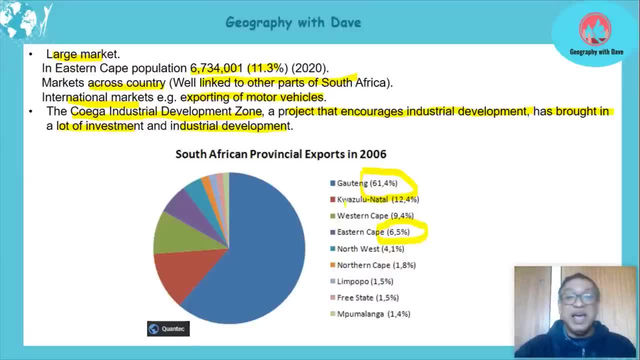 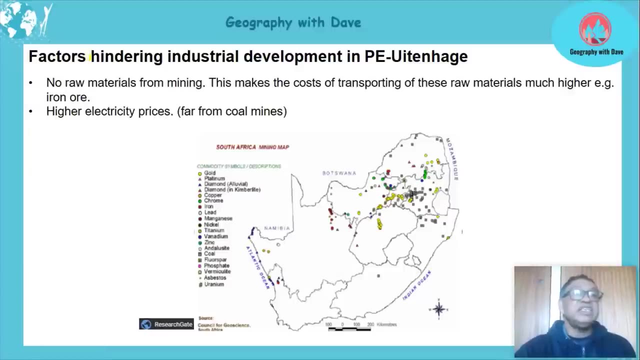 percentage in relation to how ten down here. all right, it's. i know it's much smaller, but it's still very significant. so markets, exports etc. and harbors played its huge part in relation to that. all right factors hindering no raw materials for mining. okay, no raw materials for mining or limited. 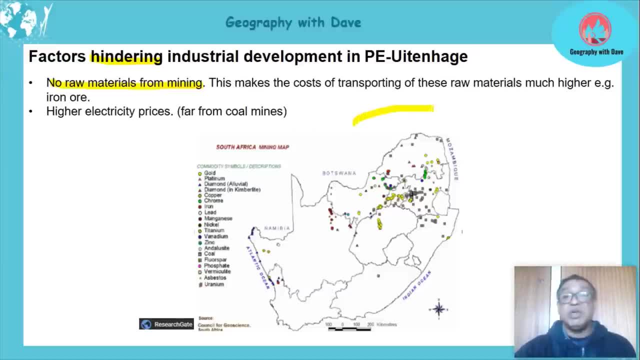 right now. look at this from mining, rather look at this, look at where the minerals are. our learners look at this. i mean, if we look at this map, all right, all these minerals are there not? not east central part, etc. and look at this area here has got no symbols relating to this. 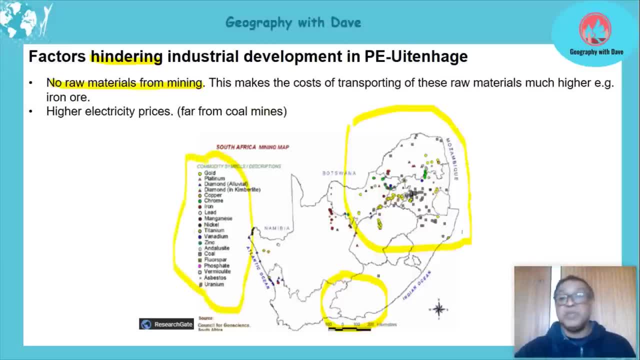 this is a definite factor hindering all right, and we need it. we need iron and steel, etc. we need iron ore rather to produce iron and steel to produce things for the motor vehicle, etc. and what does this do learners? the cost of transporting these raw materials are much higher. example: the 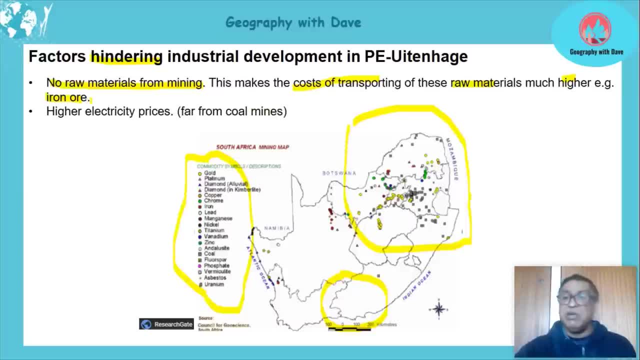 iron ore, etc. okay, much higher. or even processed iron and steel. okay, right. and another thing here, learners: coal mines, which is a major supplier in terms of the production of of electricity in our we got coal powered electricity, which is the majority of our electricity. now what happens? we far from the coal mines, which makes higher electricity prices massive. 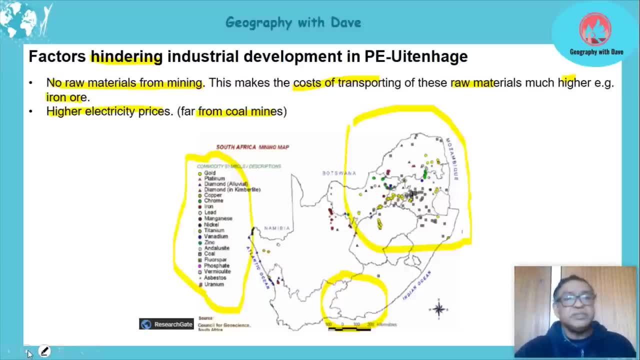 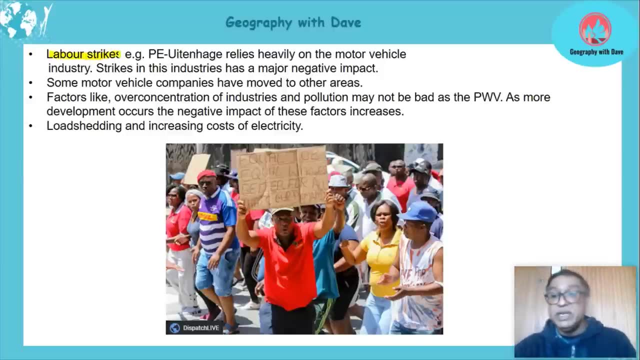 you understand. okay, labor strikes: it seems to be on a slow down at the moment- i stand to be corrected- but at least this is improving. not many labor strikes happening at the moment, you understand. uh, that's a good sign. as i say, i can't read all the newspapers. i tried to take the news. 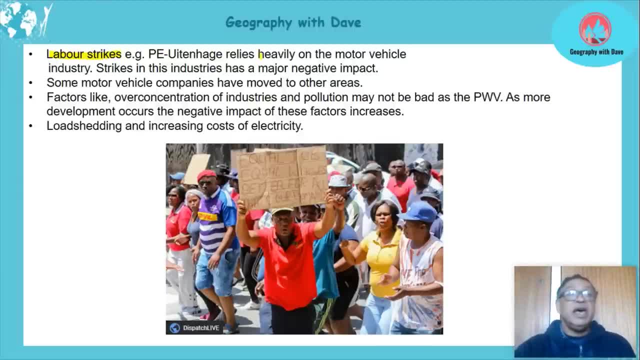 but labor strikes- and it has been big in this motor vehicle industry. can you see people striking, not happy, and of course they have their valid reasons etc. pay conditions and things all right- and it has a major negative impact. in fact, millions are lost each day. when there are strikes doesn't mean the routing, does not. 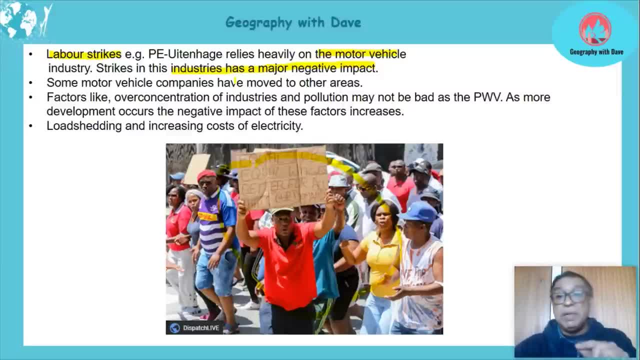 strikes, but this one has at times crippled in past years, crippled the moto industry which is huge in, uh, the peu tenague area. some more vehicle companies now have moved to other areas, i suppose because of better conditions. can be related to the strikes. all right, maybe the cost of the raw 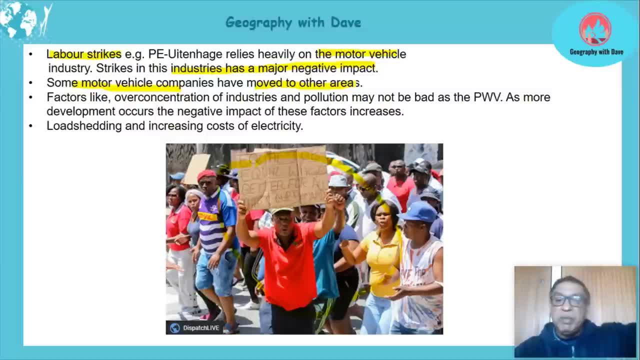 materials. okay, that they can get it cheaper, maybe in houting. so what do they do? they move to houting. maybe the costs are cheaper. okay, although the port is there. maybe they weigh the costs and say, hey, it still may be cheaper for us to move because transport has been improving. 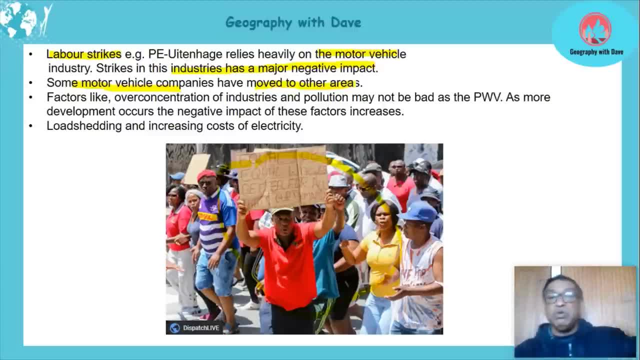 between houting and harbors so it's cheaper for us to go to. okay, so they may decide: no, i'm moving. so this is negatively impacting on the uh uh industrial development in uh the peu ten hague area, and then factors like over concentration of industries. pollution may not be as bad as the pwv, but it's still happening. 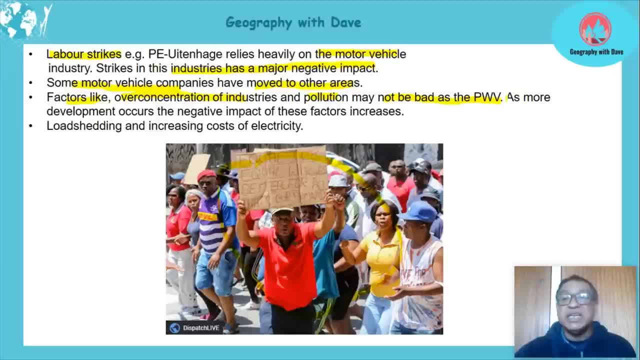 okay. and as more development happens, learners okay. as more development occurs, the negative occurs of impact of these factors increases, as obviously you understand. uh, when the area develops there will be more over concentration of industries, resulting in the pollution same effects that gauteng is feeling all right uh, in terms of those things, okay uh, traffic congestion and 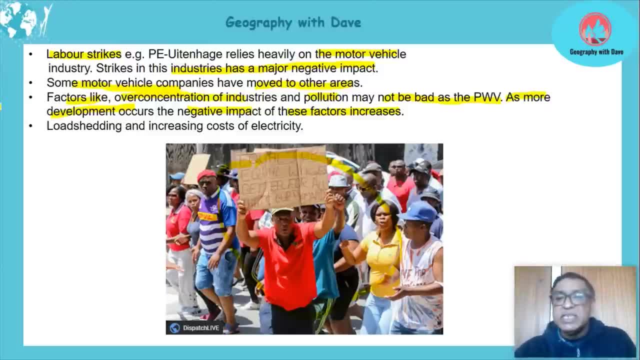 strain only. so it's going to happen, and there is a certain amount of this problem existing in the uh pe uteneg area, but not as bad as gauteng. and of course, load shedding and increasing costs of electricity uh will create problems. all right, but these are your more major factors, as i pointed. 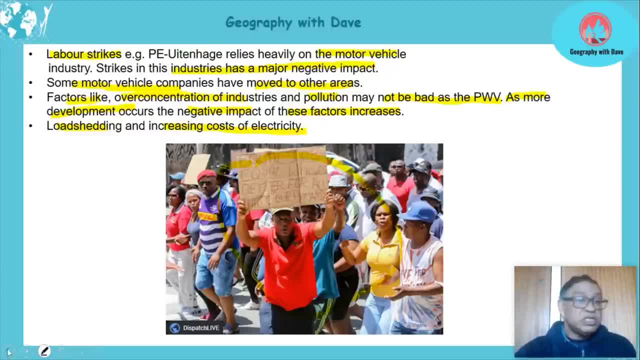 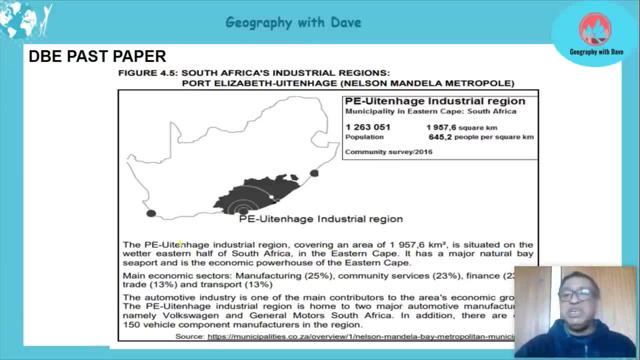 out to you earlier. okay, so certain things are similar to the gauteng region. now, obviously, we need a past paper and i've used last year's paper and i want to show you, you know i two reasons why i use last year's paper. uh, learners, it shows you. 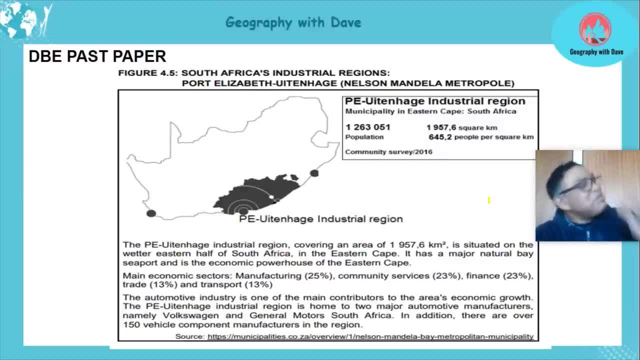 the value of a resource and how simple you can actually pick up certain factors. okay, sorry, sometimes i'm looking, i'm looking at the clock to say i can't take over my time, otherwise we won't fit this lesson in a lesson. eh, all right, so let's look at this. this is a little uh. 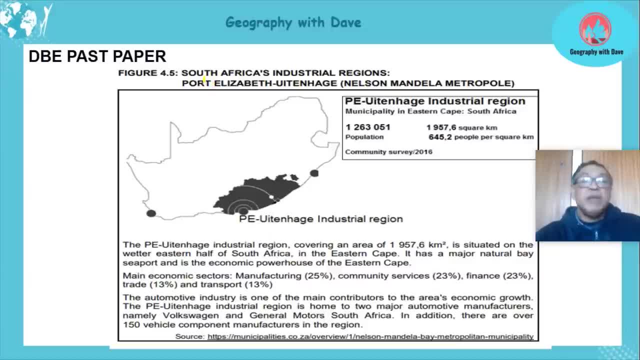 practical. okay, right, i'm going to get. there's another word that it's called. you don't get worried, i'm going to show you that word just now, with a little map information and it says: South Africa's industrial regions, the port Elizabeth you'd make, that's the Madison Mandela it gives. 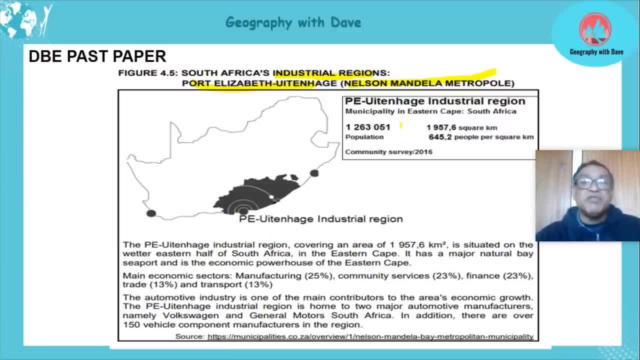 us some indication here. don't forget, read every bit of information. it tells you the population. can you see it's huge. that is why I didn't want to give you, uh, the population of the area, because I'm showing it to you. can you see what the examiner has done? they didn't give you for the Eastern Cape. the figure is different. 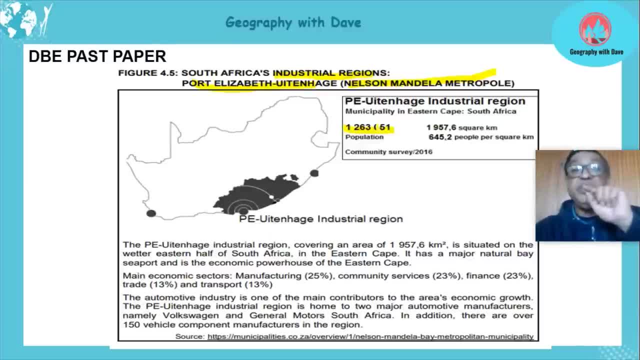 because it's now specific to the PE uterine industrial area, and that's what I'm talking about. learners don't just learn off figures and expect that to appear. the geography has got so many things you understand. it's undergoing so much change that you need to interpret the 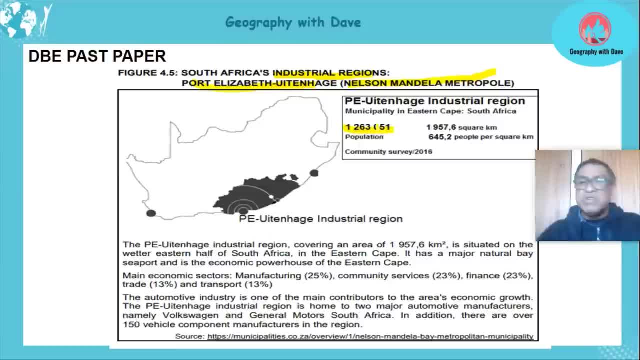 information that you have in front of you and apply to it, and you can still do it. all right, it's a large, relatively largest population for one area of a province. it covers a huge area in terms of uh square kilometers. all right, it's 645 people per 45.2 per square meter. quite 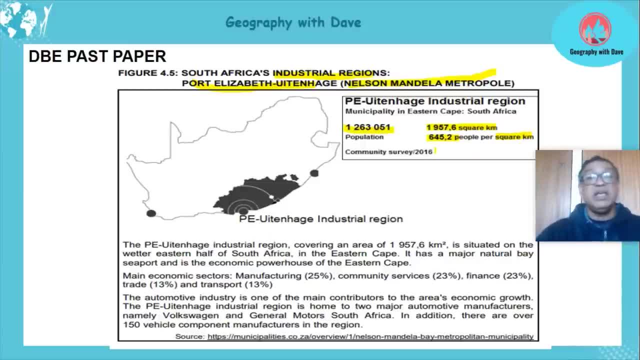 densely populated, maybe not as heavy as counting. all right, okay, and of course that's the reference. let us read further. let's take the words. the PE uterine is being referred to you covers an area of of 1956, 57.6 square kilometers. so we see it's huge. it's situated on the wetter Eastern half of South. 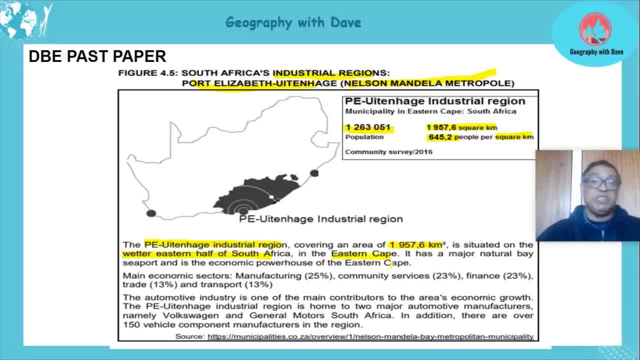 Africa and in the Eastern Cape. see what I'm doing, learners. I'm highlighting the main words. okay, has major natural Bay. why is the examiners giving us all this? it's significant learners because they most probably going to use some of it seaport and is the economic powerhouse of the Eastern 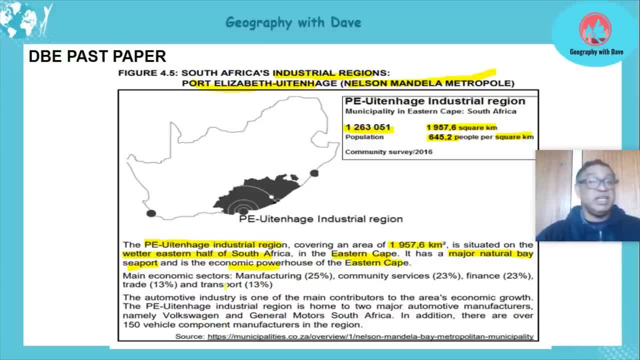 Cape tells you it's the massive area in the Eastern Cape. regarding that, it talks about the menu economic sectors. manufacturing is Massive, then it's Community service, then it's finance- okay, finance- and then it's trade and then it's Transport. can you see manufacturing, all right, massive. 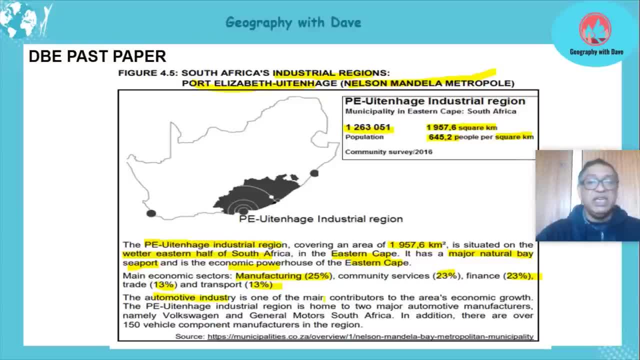 the automotive, the vehicles, eh, is one of the main contributors to the area's economic growth. why is the examiner picking on the automotive or the motor vehicle industry? all right, most probably something is going to pop up, eh? why just remember the specifics here? okay, that's how you read, that's. 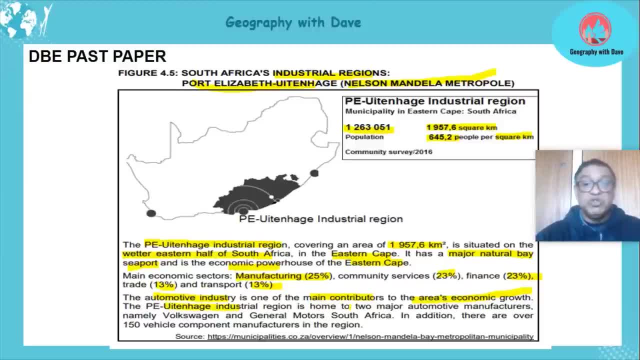 how you get it. the industrial region is home to two major automotive manufacturers: Volkswagen and General Motors. all right, South Africa, okay, and in. and there are over 500 vehicle component manufacturers in the region. I can see without looking at the questions. all right, examiners are nice people. all right they. 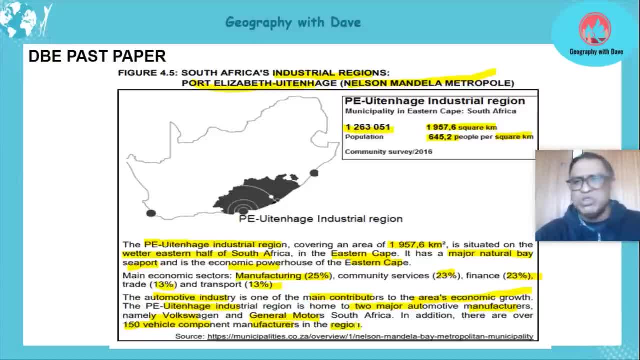 give you stuff that you can use. they won't give you a hundred thousand facts. not all the facts will be quite certain things that you need to use. okay, so we've got an idea already of the questions. eh, that's the brilliant part of trying to work the source and you actually work on questions. okay, why are? 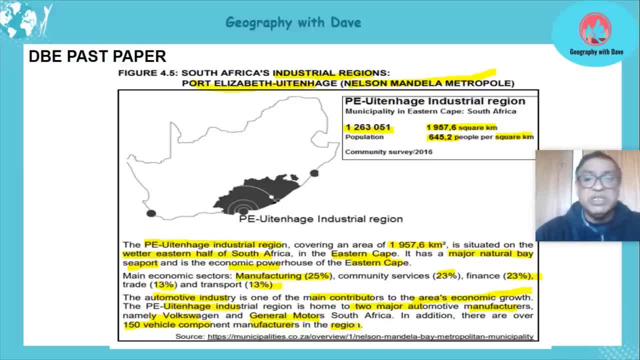 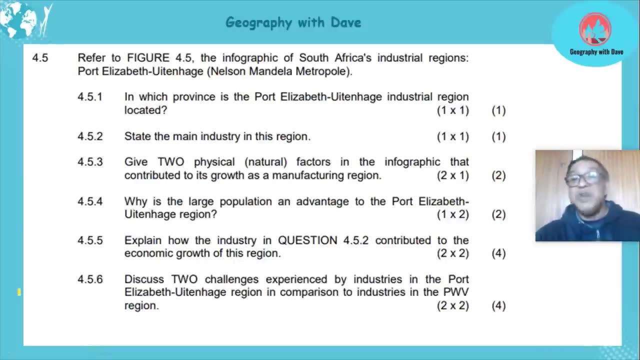 they picking on Eastern Cape? why are they picking on the motor industry? why are they picking on the natural seaport? you understand why is these things being picked on? okay, so let's look at the questions. this time I decided not to put in the memo because I want to work with you that you can think also. 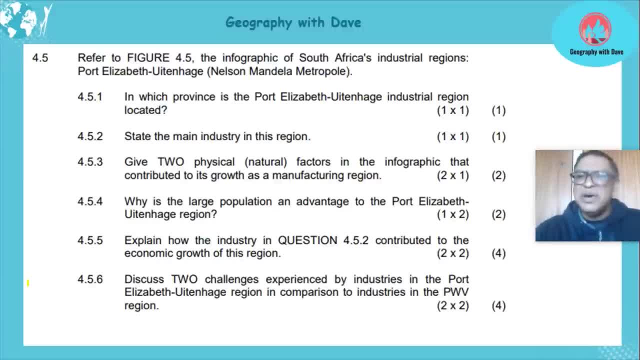 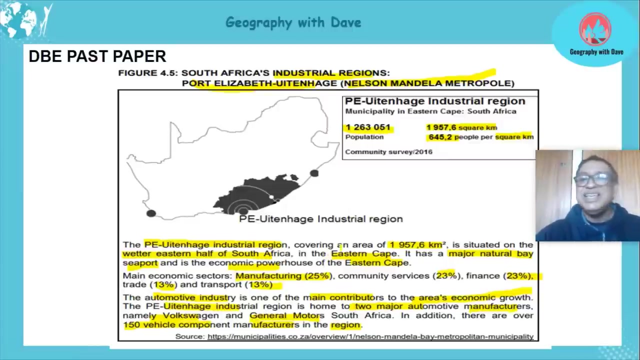 sometimes the memo is just: let's work through it together, learners. all right, and look at the article. the first question. all right, uh, which province in the Eastern Cape or Port Elizabeth, Utinake area industrial area is located? all right, and there, if we go back to our article, beautiful, it's in the 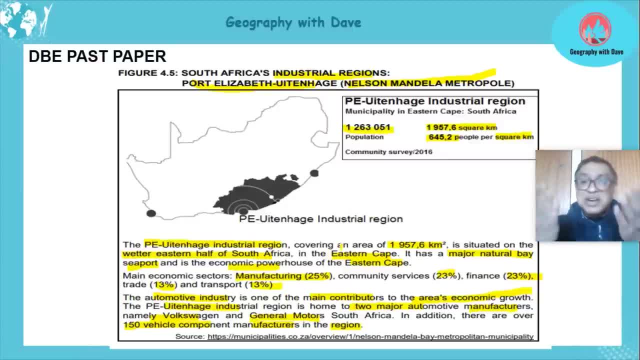 cake. can you see learners? all i had to do was read through this, okay, and i've got an answer already. brilliant. i'm not saying all the time it's going to be like this, but you will get occasions when it is like this. this is easy marks. it just means reading. okay, let's go on. 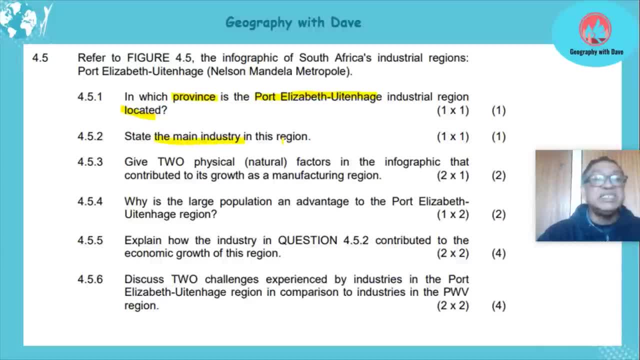 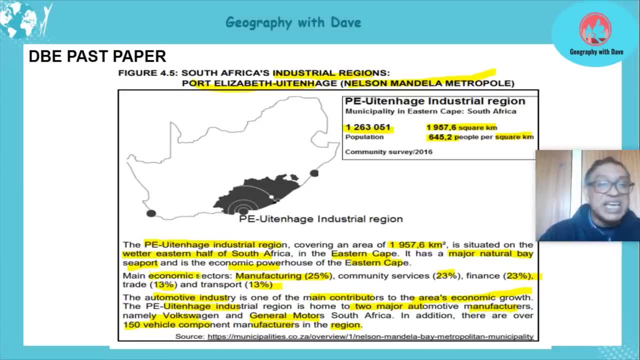 let's check the second one state: the main industry in the region. all right, let's go back now. watch out. remember this is economic sectors, and in this exam some people are writing manufacturing. but what does the examiner want? the main industry in the region, all right. and of course that's your automotive industry, can you see it? all right. so sometimes you have. 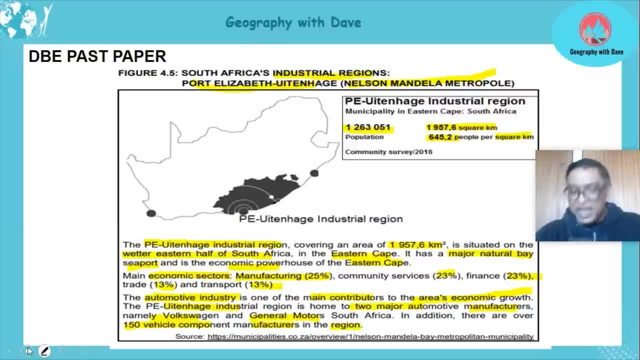 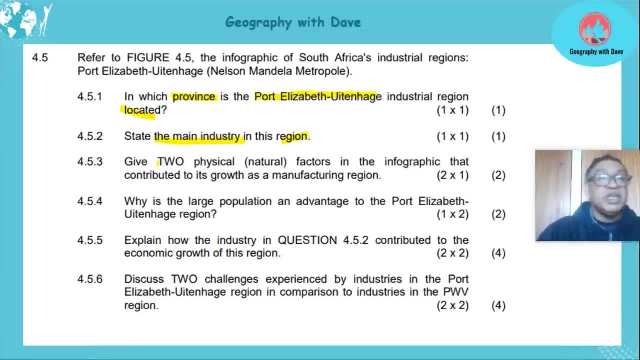 to be careful learners, just be careful. the answer is no there, but sometimes you may just take the first one, read carefully, all right, let's the next one give to physical, which is natural factors reading these words. hey, no selective reading where you say: give two factors, read properly, all right. can you see the word in the infographic right now? i haven't. 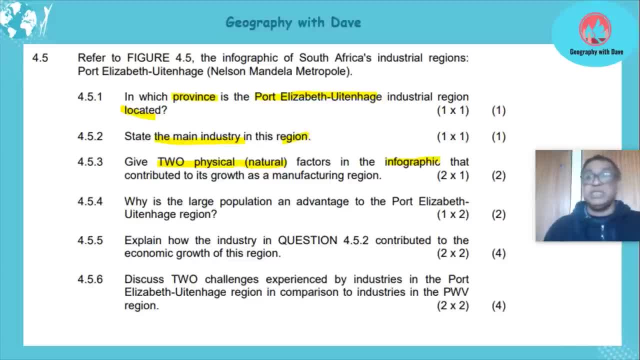 touched the word infographic. sometimes maybe teachers are teaching with sketches, so what you understand, that's the infographic. it's giving you diagram information, etc. or map information, etc. it's called an infographic, so don't get confused by this. that contributed to the growth of the manufacturing region. it must come from the information there. okay, must come from the information, all right. 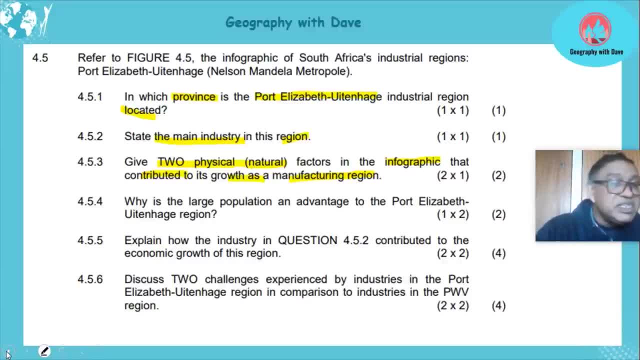 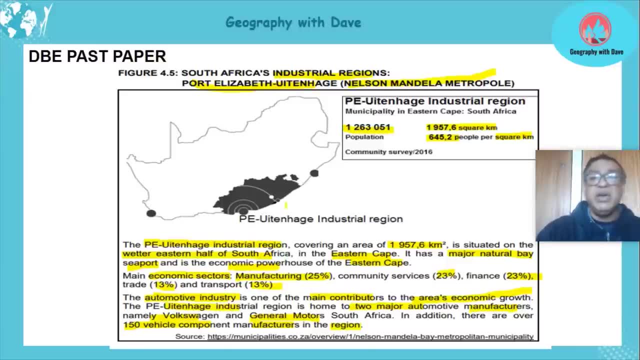 now we go back to the information learners. let's read. it's given information. yeah, all right, it's given information. yeah, okay, right now let's read here: can you see the wetter western part of south africa, so it's a natural thing which is rainfall, isn't it? the wetter part? enough water supply? okay, it's on the east. that's one factor. let's go on. 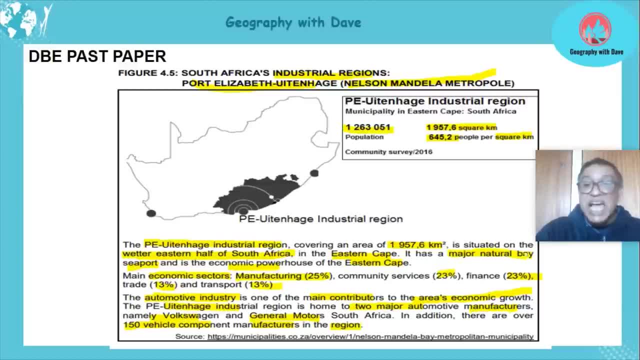 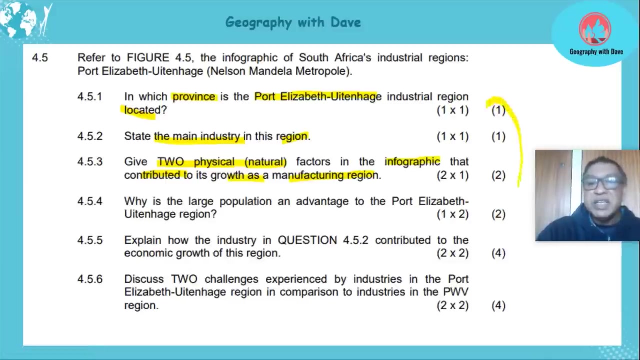 and the examiner's made it easier. major natural bay: okay, seaport, all right, can you see it right there? it tells you those are your two natural features. so at the moment, learners, what has happened? four marks is just there, just taking and putting. all right, if you. 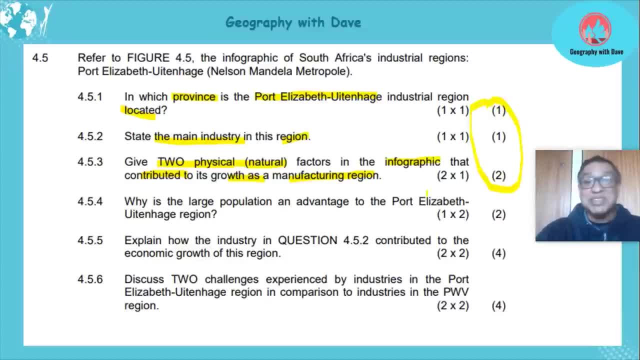 look at it: four marks- that's a lot of marks for a section which is actually that's ten and a half. six is a three mark. that's a lot of marks for a section which is actually that's ten and a half. 14 months, four out of 14. so please get these resources and check them. why is the large? 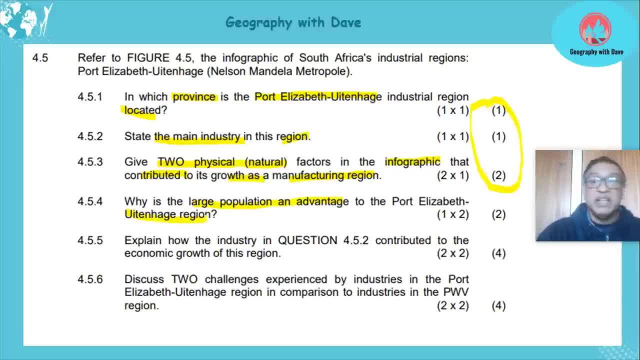 population an advantage to the uterine area. okay, now you have to take it a little further. learners, you've learned already. what does large populations do? okay, it gives them a labor supply, isn't it? you've learned this. and it's not that we call it a little middle order, etc. but doesn't? 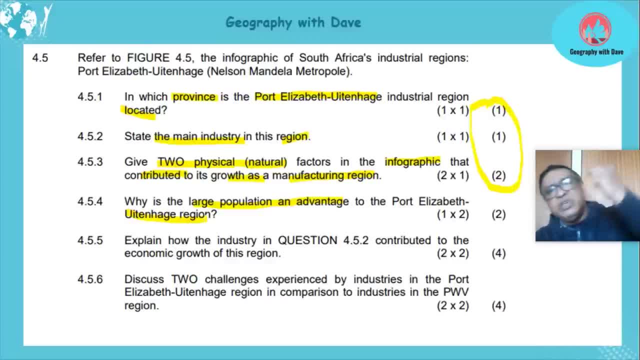 mean it's difficult if you know how to apply your work. okay, so you've learned this already. it's in the notes that it allows for sufficient labor supply. you understand that can be there. all right, it's for two marks. remember again one times. two means one fact because of the one. 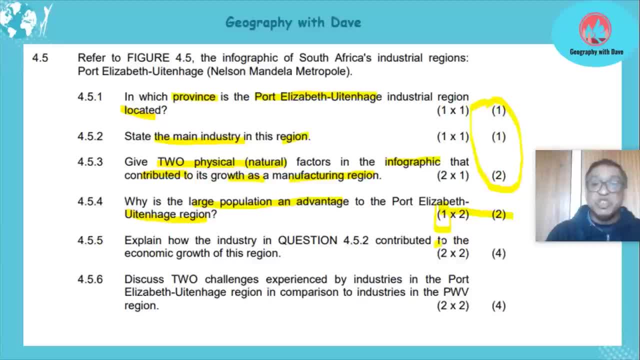 you and you have to explain it properly. and two times two means two facts, fully explained, okay. and then, if that's your major factor, then if you've got a large population, don't you have an immediate market to buy your goods? wouldn't that encourage, uh, industrial development? okay, you've got a million. 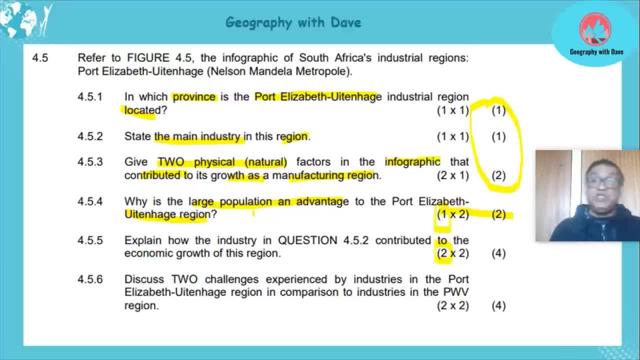 people more, whatever, and people are ready to buy your goods. brilliant, you understand. then it says: explain how the industry in 452- remember, read these things, learners. 452 is talking about this industrial region. the automotive industrial contributed to the economic growth of the region. all right, number one. i know employment can be uh, economic and social, but yes, 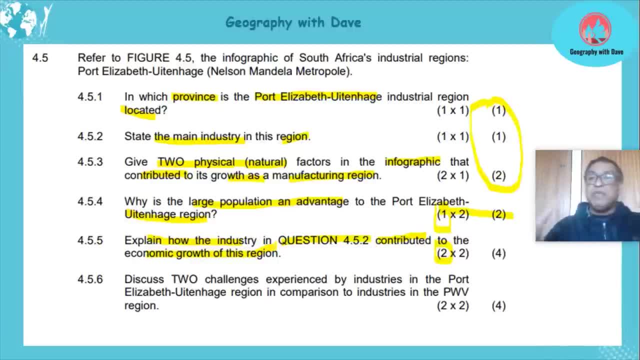 the motorcar industry employs a lot of people. all right, therefore, creating massive employment whereே social benefits, creating massive employment related to the motor industry. don't say a lot of employment, because it says specifically to 452 learners: which is your automotive industry. automotive industry needs people, significant amount of. 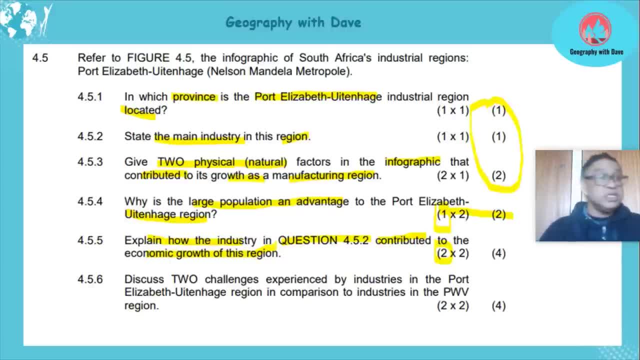 people, a lot of people to work, so therefore it creates employment. all right, uh, we need to transport goods from the automotive industry, not produce your начал to self-employment. appreciate it from the there. we need to have, uh, infrastructure, power lines, etc. so therefore it improves. 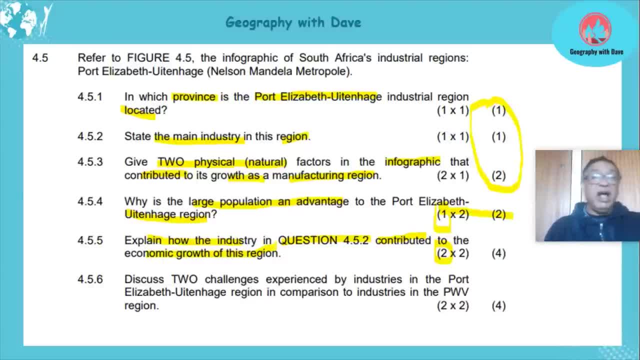 infrastructure, okay, uh, for the area. can you see how i'm doing it? learners, all right. uh, in terms of that, of course, because it's a large with the infrastructure. the next point: it will encourage more investment in the area. can you see how i can go through this all? 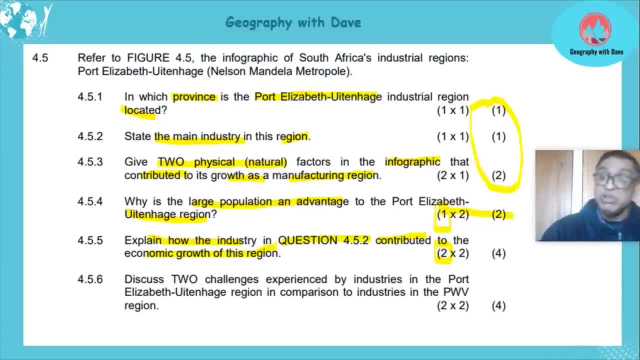 right. the memo may have other facts also, but my facts is good also. you understand all right because it's related, but please note, related to the industrial active, uh, industry- that you chose the automotive because it says four, five, two. is that clear, learners, don't forget, don't just write. 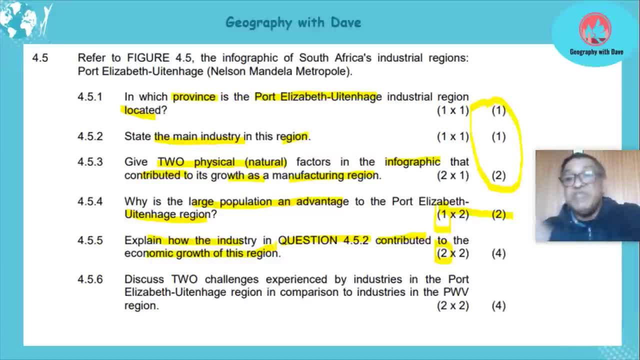 more employment. say what the automotive does. it employs large number of people, thereby increasing the employment of automotive industry. okay, state discuss two challenges experienced by the port elizabeth region in comparison to the pwv region. be careful, this is a compare question lettuce and we have to compare. okay, don't just say it has small. okay, i know you may say you correct. 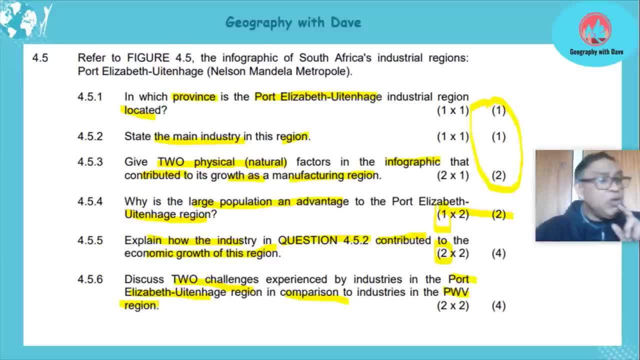 but put it in full: okay, uh, one things uh. compared to the pwv region, the pe eutonic region has no raw materials relating to mining or has no mining raw materials which affects the production, because you need that iron and steel. okay, uh, coal mining- nothing in the port elizabeth. 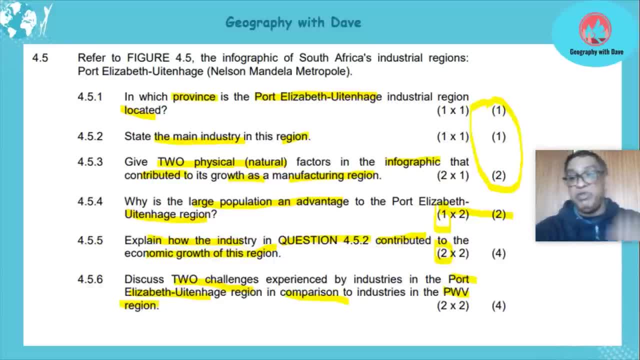 region. okay, compared to the pwv region. can you see what i'm doing? maybe the examples will accept it in the other way, but let's not take a chance, as you say, no tatama chance. okay, so we say: compare it to the pwv, which is a lot of coal mines, you understand? therefore, the 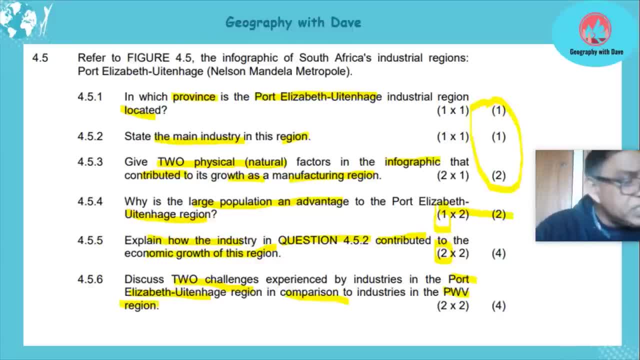 Electricity will be expensive. okay, I can use other facts also. If we've got our four marks, which is the main ones, I could use other facts. In fact, it's away from compared to PWV. it's further away from the rest of Africa. 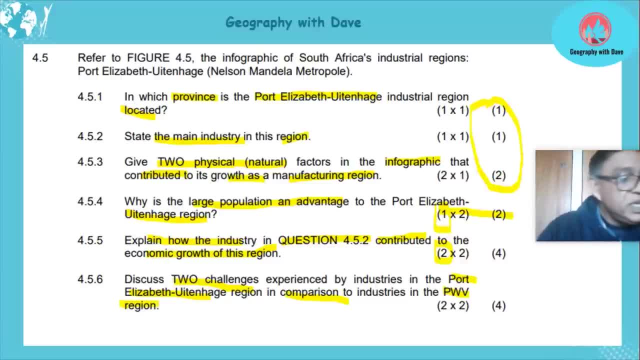 So Africa trade may be limited. You understand, I could use even not smaller points, but that doesn't mean it's insignificant that there's less tertiary institutions et cetera. Can you see? it's about applying learners And that is the important thing. 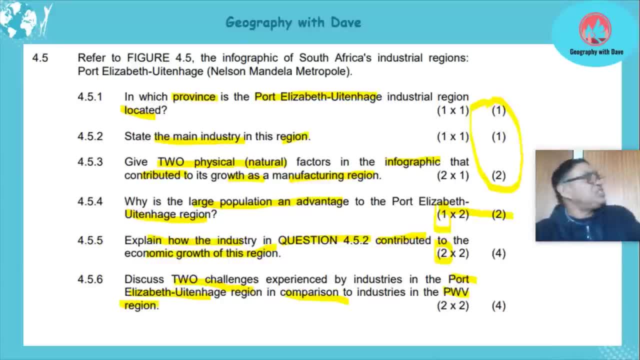 And you can never get it wrong. They'll bring any information to you relating to these issues, anything. You understand Different resources, but you'll be able to apply yourself. Okay, learners right. This, then, covers the four core areas with regards to our curriculum.